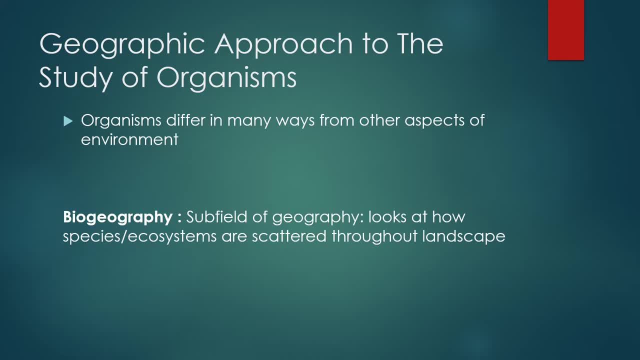 found across the landscape. So you know, geography is a very broad discipline, right? So we're going to kind of apply this geographic approach to the study of organisms, plants and animals. okay, So organisms can differ in many ways, And there's this subfield of geography which is called 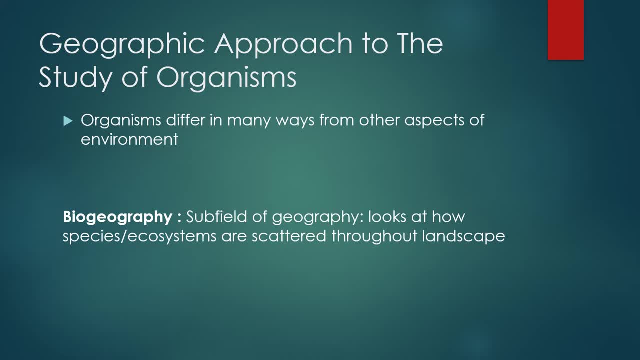 biologics, Biologeography, one of my favorite topics and disciplines under ge. Good morning, My little doggy just woke up. Hi, He's like an old man, Choo-choo. What is she doing? Choo-choo You guys. 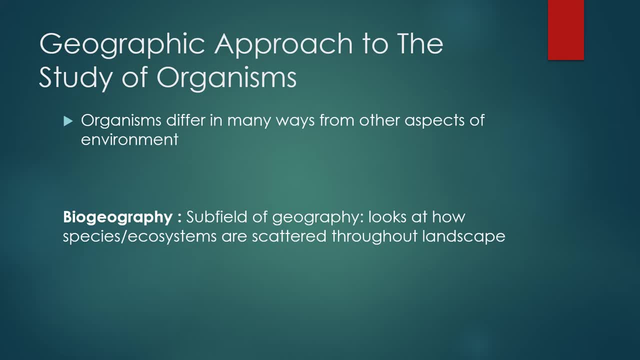 just heard my dog mom voice. Want to go outside? Huh, But geography is a field of geography looking at how species and ecosystems are scattered throughout the landscape. So if you remember, in the beginning of the semester I said that geography we take like different types of. 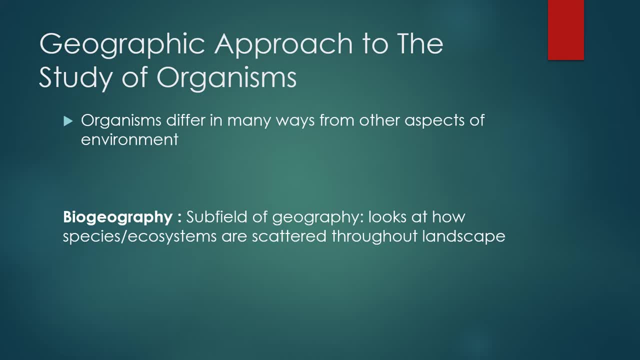 information right, We make them more understandable or we find patterns and similarities, right, And you kind of break that down. So we looked at the different spheres, the hydrosphere. Now we're going to be looking at specifically the biosphere, all living things, So the term biodiversity, 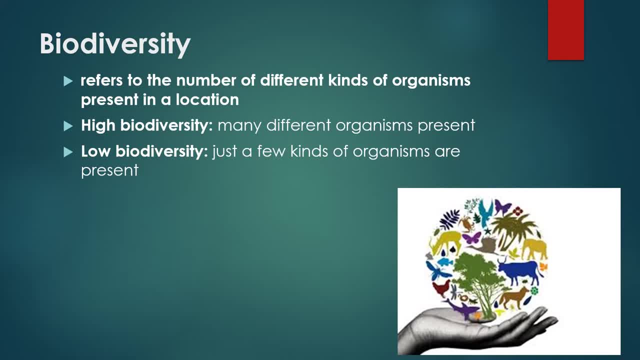 which means Biological diversity. It refers to the number of different organisms present in a location. So a place can have very high biodiversity, A lot of different types of organisms are present in that area, Or low biodiversity, right, And so you don't have a variety of organisms, Not really a. 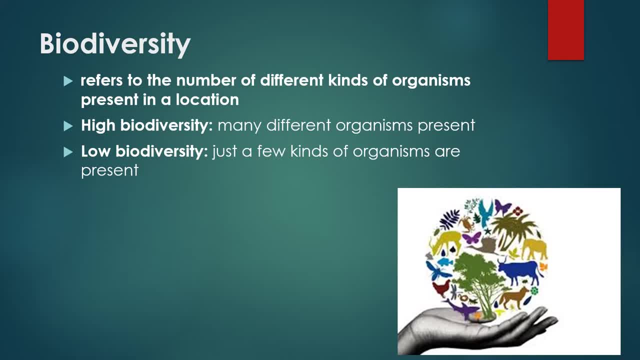 lot, but just not a variety. So if we were in the classroom I would ask: okay, class, where do you think you would find high biodiversity? You guys would be like, oh, probably the rainforest. You're like, yeah, you guys are really right. Yeah, the rainforest, a coral reef, those places. 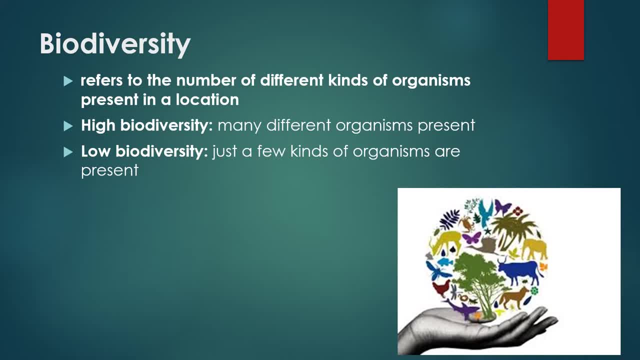 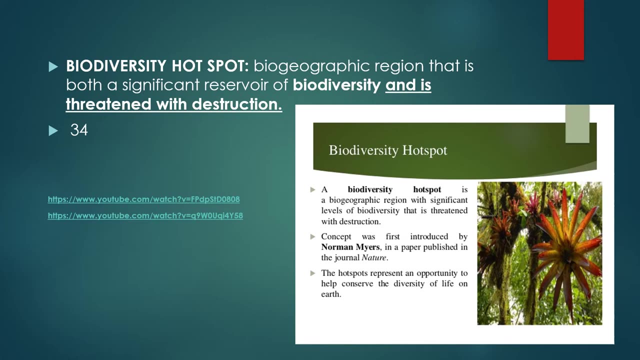 those have high biodiversity, right In places like urban landscapes, cities, deserts, the tundra. these would all have low biodiversity. So when we look at biodiversity, there's a term called called biodiversity hotspots, which describes different places on earth that have obviously 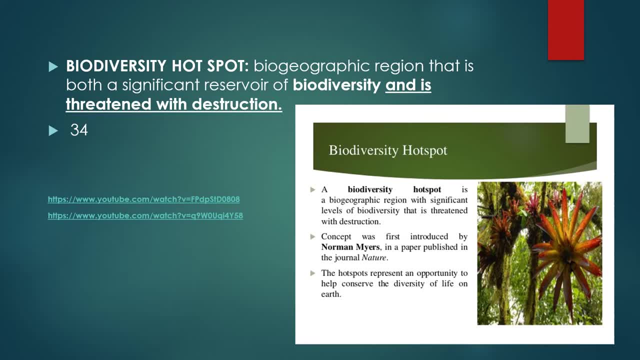 high biodiversity but at the same time, they are threatened with destruction. So it could be because of climate change, It could be because of land use. Most of the times it is because of land use. So many different reasons that are threatening that location and its existence makes 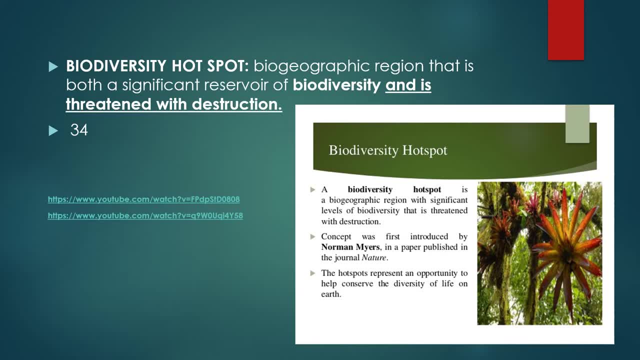 and has high biodiversity, makes it a biodiversity hotspot. A biodiversity hotspot is a region with significant levels of biodiversity that's threatened with destruction, So this would be by the hand of man, specifically right. So this concept was first introduced by Norman Myers. The hotspots represent an opportunity for us as scientists or educators. 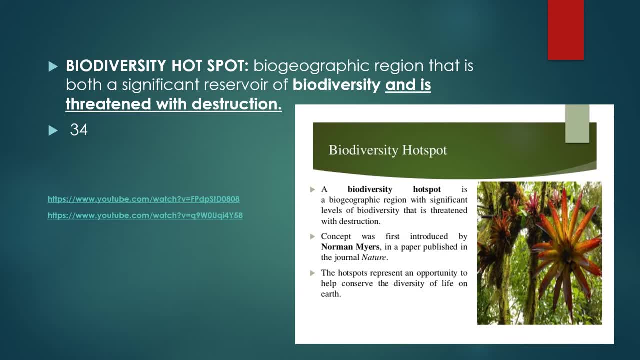 really to highlight this area and hopefully save this place before it is completely eradicated, Right? So currently there's 34 of those on earth. So you have to remember: yes, they're beautiful, but at the same time, it's being threatened with destruction. So that's why. 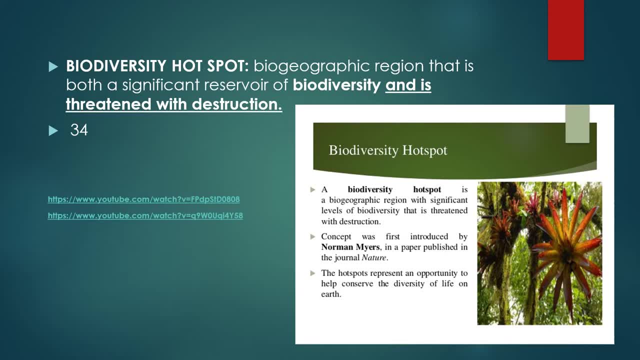 they're getting this kind of like more, I guess, more infamy, right? So I'm going to choose two, two of them out of all the 34.. This has different places on earth. Obviously, we think of rainforest. 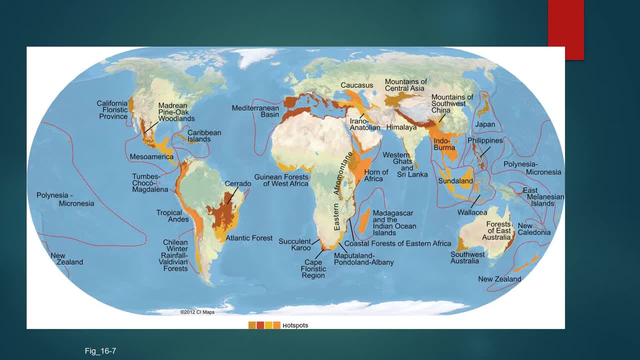 Yeah, The rainforests are probably going to be really threatened, right, But there's other places. I mean, look at California. Is it surprising that we are a biodiversity hotspot way over here? California, Los Angeles, is a biodiversity hotspot. Crazy, right. It's not something you would imagine to be a biodiversity. 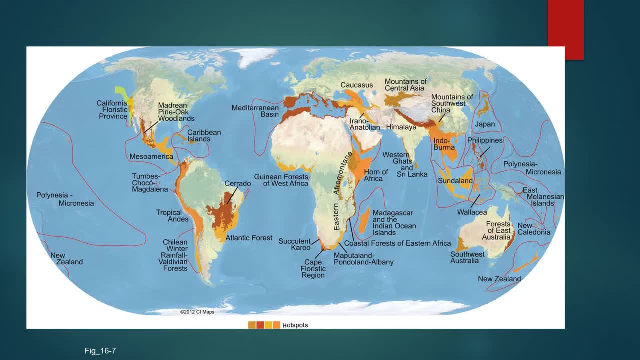 hotspot. So I'm going to be highlighting the California Floristic Province and this area here. okay, The Lazer Ecosystem, But I mean these are all hotspots all over the earth. The California Floristic Province it does include. 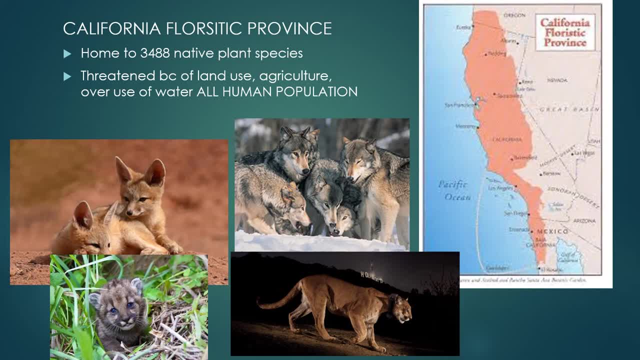 the Chaparral Environment which I talked about in Chapter 8, but it goes a little higher and it extends a little more than just our Mediterranean Climate Zone. The Mediterranean Climate Zone, yes, it is included. It's probably all this area here within this California Floristic Province. home to about 30,488 native plant species. okay, So here in California you have all these different things working together. You have a lot of geological activity, earthquakes, faults, which give us our rich soils right, Which bring in the diverse plant life, which then bring in the insects, and 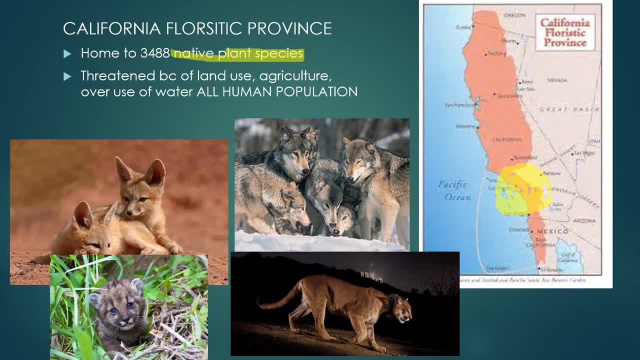 then bring in all these different types of endemic species. You have that coastal area, You have mountainous mountain ranges, You have the Central Valley, which has this fertile soil- I mean there's a lot of things going on- and you have all these different climate systems. Up North it's going. 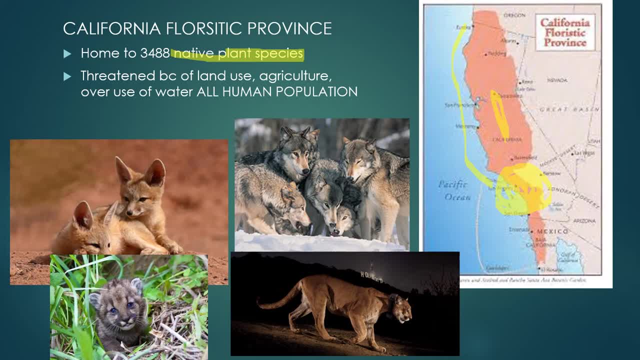 to be a little bit more rainy. Down South it's going to be drier, but you do have, you know, mild winters. So it gives us all this diversity right. The California Floristic Province is a biodiversity hotspot, one of the only biodiversity hotspots in the developed world. California Floristic Province is a biodiversity hotspot, one of the only biodiversity hotspots in the developed world. 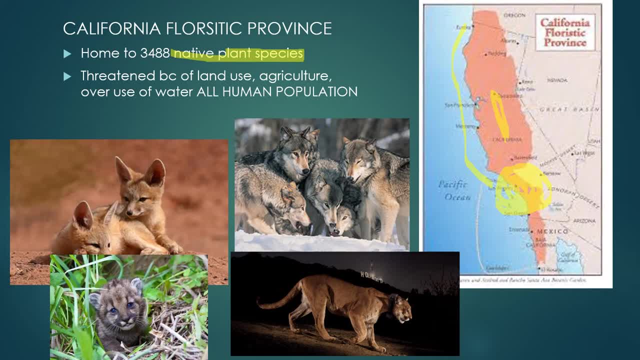 world. That's crazy, right? And yeah, of course it's threatened. Why is it threatened? Well, that's easy, because of land use, agriculture being the main reason. right, We got to feed all these people, but the main driver is going to be human population. So here's just some of 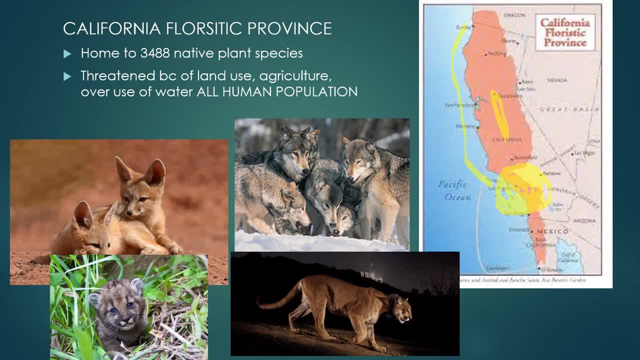 the animals that you would find that probably are currently threatened. This is the California- no, sorry, the San Joaquin kit fox- So cute, right- Our California mountain lion, then grown up over here, and our gray wolves. So I think a few weeks ago we did watch that gray wolf. 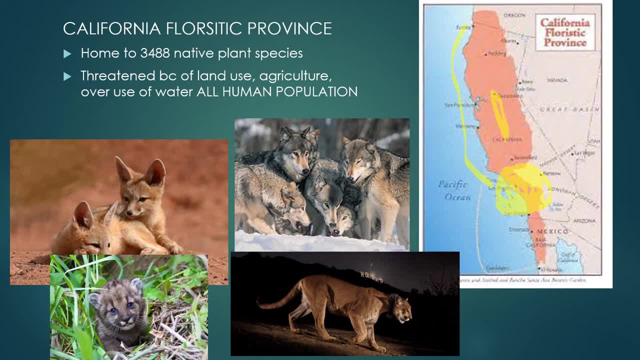 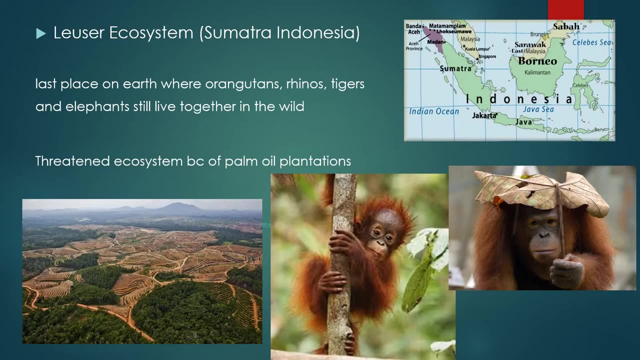 video and how the reintroduction of a top predator will bring the ecosystem back to life. Right. So California, for a floristic province here where we live, is a biodiversity hotspot. So diversity hotspot is going to be something more of what you would imagine, which is the 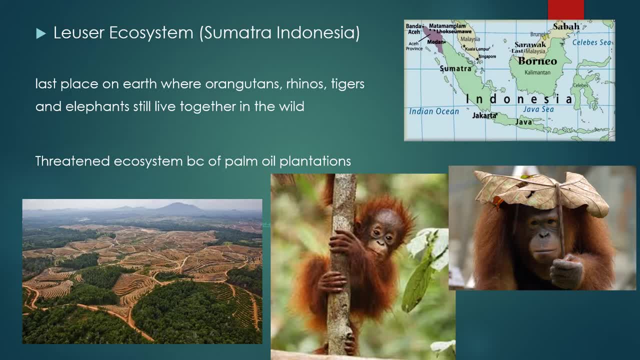 lazar ecosystem found in sumatra, indonesia. so if you look over here, this is where it's located. um parts of sumatra, borneo. this is all indonesia, um a different collection of islands right underneath, um thailand, cambodia, right. so this collection of islands sits right at the equator. 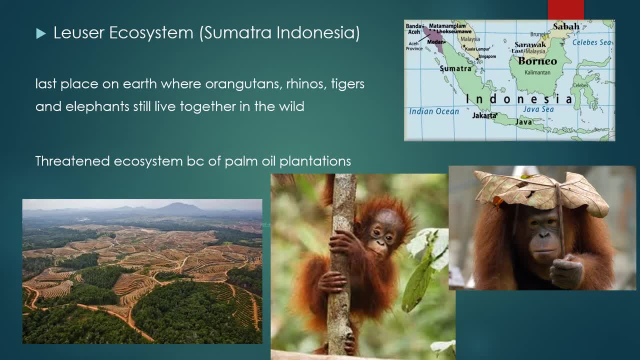 huge rainforest. this is the last place on earth where you find orangutans, rhinos, tigers, elephants still living together in the wild right. so that's huge, but it unfortunately it is threatened and i know you guys watched the um racing extinction video and they did talk about it a little bit. 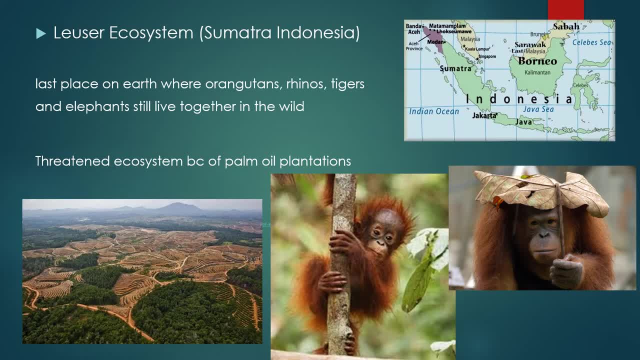 um, so these orangutans are critically endangered? first of all, i mean: look how cute they are. right, some people don't think they're cute. i think they're adorable. some one of my favorite animals. they are closest to us in dna. um, they're very, very smart. they also live with their 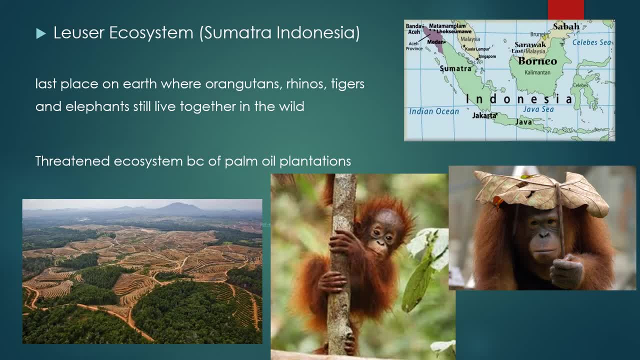 mom, i think up to 13 years. i want to say it's 9 or 13 years, which is the longest out of any animal in the animal kingdom. sorry, i had to pause it there. um, yeah, so they stay with their mom the longest out of the whole animal kingdom. and so what that means is that when 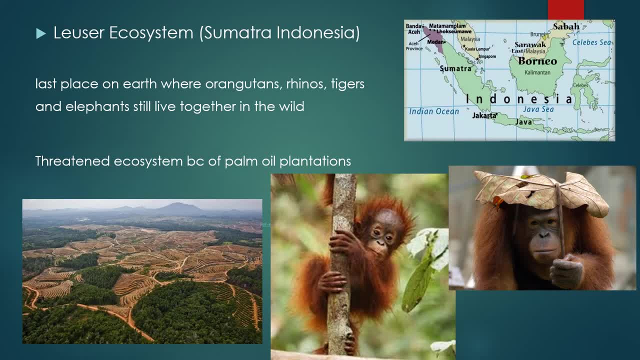 they leave, um, they come back and they visit mom, so they're really like this um really tight-knit family, and they spend most of their lives in the trees. so what i'm getting at is in indonesia, there is a huge threat to the environment because of palm oil, so palm oil is a very cheap commodity. 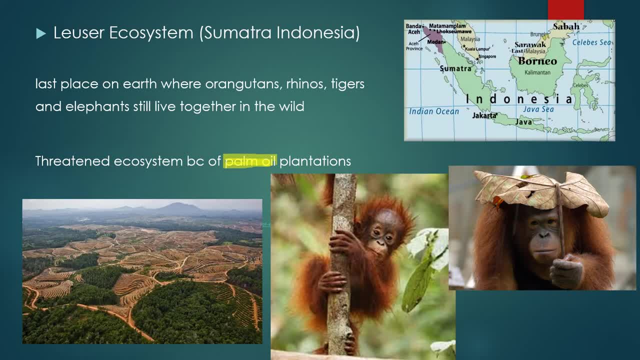 it's used in snack foods, it's used in detergent, it's used in almost anything, as a stabilizer or just this really cheap ingredient, um, just like a vegetable oil, right? so instead of using vegetable oil, we are now switching to palm oil, because, number one, it's cheap and it's not produced. some. 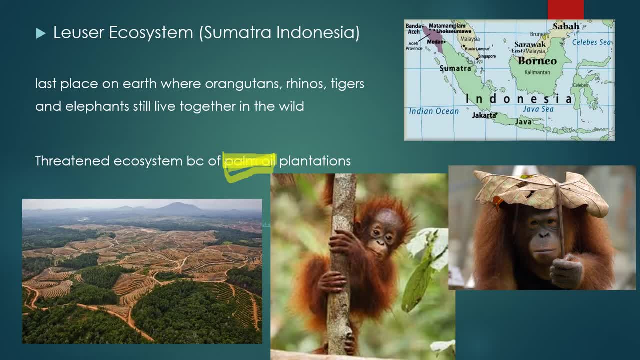 of most of it is not produced here, so in the, in this area, it's a very cheap commodity. so what they're doing is they're taking out the rainforest, clearing it, and when they clear it they don't like chop down the trees. um, they burn the area and then they plant these palm trees, and then they. 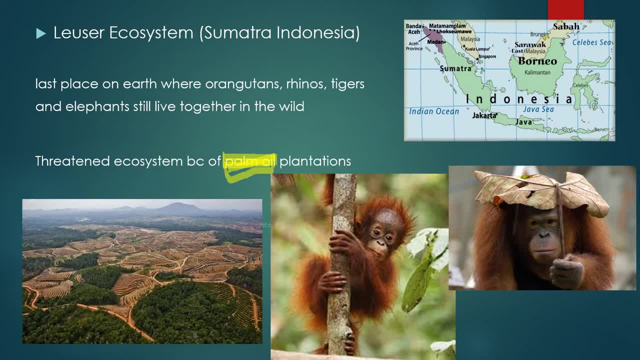 care. they give out this little tip of some sort of plantable oil in a spray bottle, so that those vegetables or fruits are actually called palm tree plants, which basically is palm trees plantation style. so they're just rows, infinite rows of palm trees that give out this little, like this little. 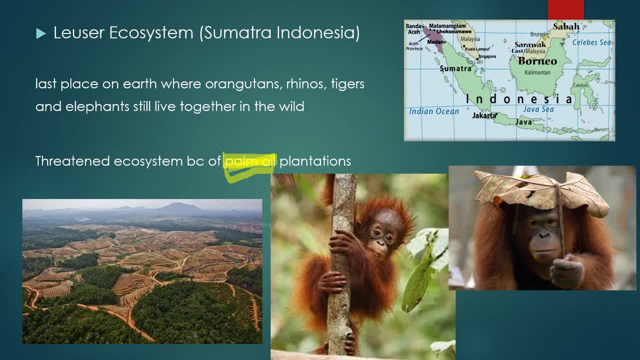 orange ball. they should really learn the name to this. but it comes off the tree. you expel oil from it and turns into palm oil, so that palm oil is used for the snack food company. i mean makeup, you beautiful, beautiful animals. and a lot of times, 90% of the time- these loggers come out and they 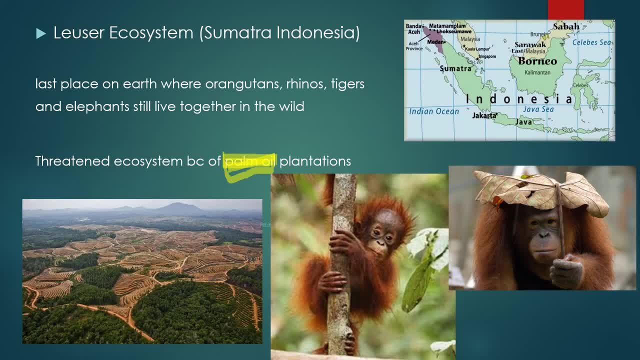 take down the rainforest and you find dead orangutans, the moms and the babies clinging to them. so there are, you know, these conservation groups and sanctuaries and non-profit organizations out here trying to protect and save these orangutans. but that is not the life right. 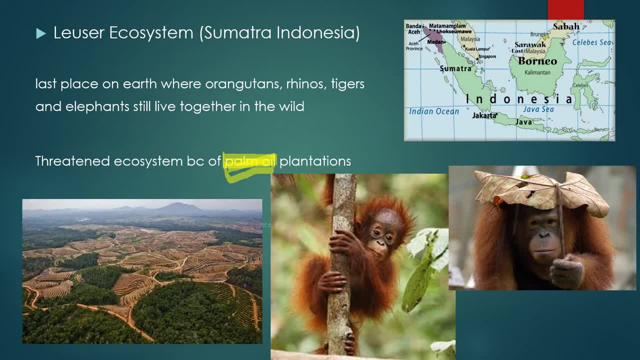 they need to be in the wild and the free. so they are critically endangered because of our snack food industry, and so I'll have a few links on your module and you'll have a few exercises, but you know there are some places that are banning this type of palm oil and you, as a 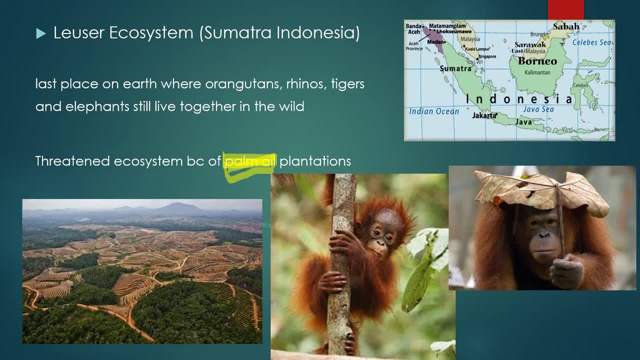 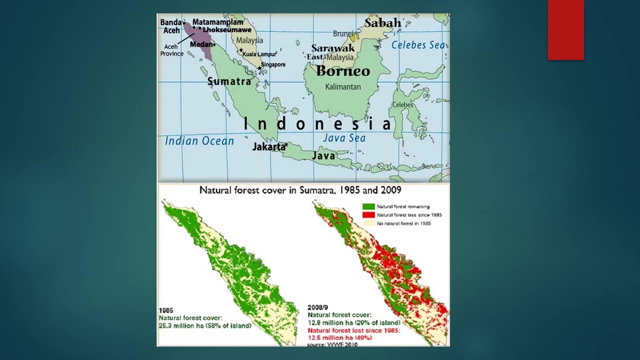 consumer, you do have the power, you do have the right to demand conflict-free palm oil. so I don't know, guys, really, really sad. so we'll see what happens with that fight. so here is just another map a little bit closer of where it's located. this is natural forest cover in Sumatra, the island of Sumatra. 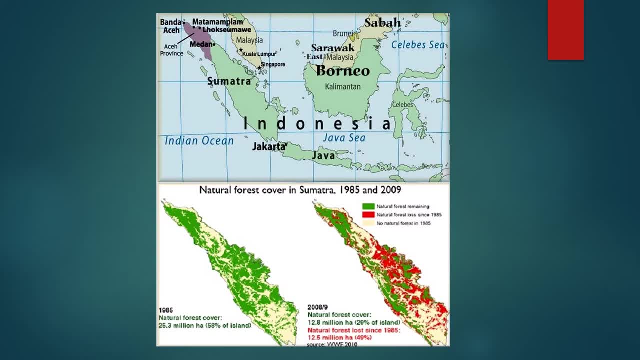 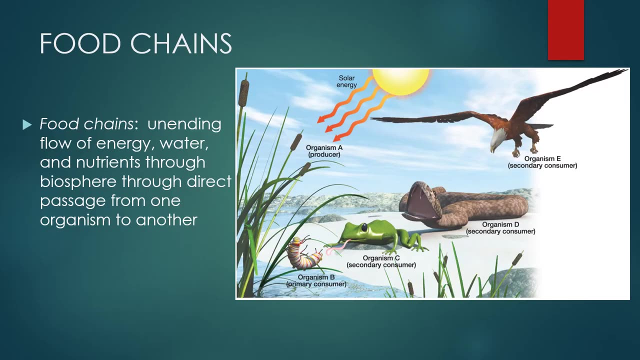 1985 versus 2009. if you see, this is you know older data, right? if you see the red, that's where it's been lost. I mean, all that has been converted into these palm oil plantations. okay, so let's talk about food chains. food chains are an end and sorry an. 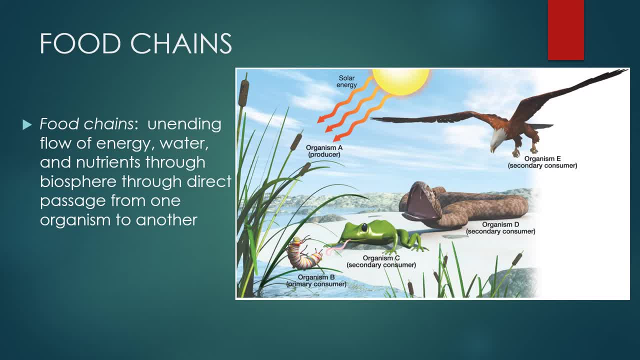 unending flow of energy, water and nutrients through the biosphere, through direct passage from one organism to another. right. so you have organism a, converting energy from the Sun through photosynthesis into a type of energy or food. organism B is a primary consumer, eats that plant right. then organism C and so on. so throughout this chain, a lot of different things are being 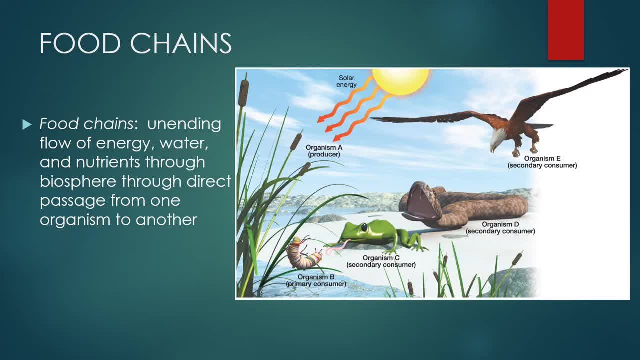 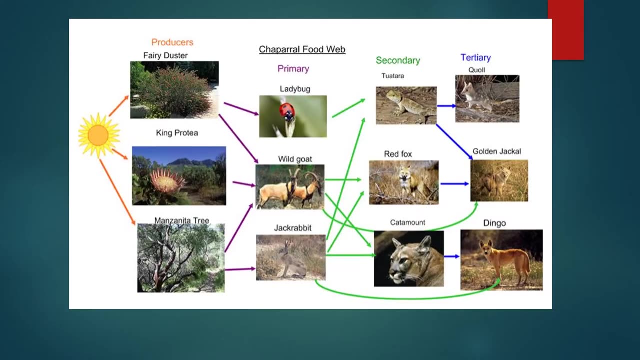 passed from, I mean through the ecosystem, right from living things, to the ecosystem, and so this is how, like nutrients, energy, water is moved from organism to organism within the Nico. so this would be a chaparral food web, and you know it's to describe a food chain as a food web, because it's not like organism A is eaten by organism BC. 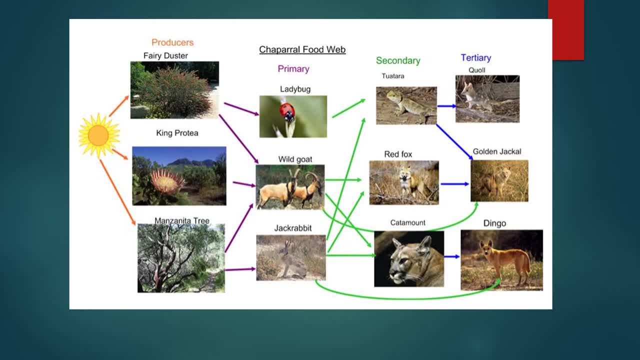 all the way back to where it's decomposed right. It's not just like this very black and white process. When you get into the secondary or tertiary consumers, things get a little bit more mixed up. There are some consumers that eat a variety of things. There are some consumers that 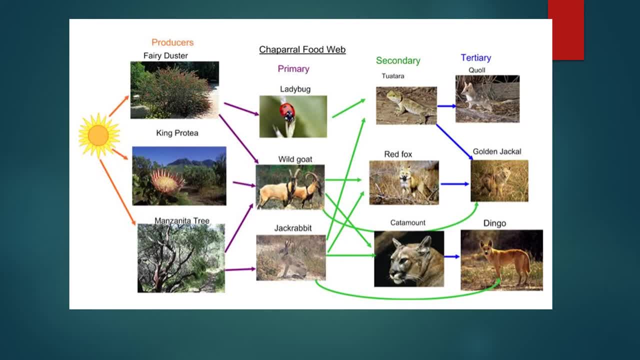 will only eat what's beneath them, right? Does that make sense? So it's more of a food web rather than a food chain. This is a chaparral food web, but remember, chaparral is found in five different places on earth in that Mediterranean climate zone, So this is not a Los Angeles or Southern. 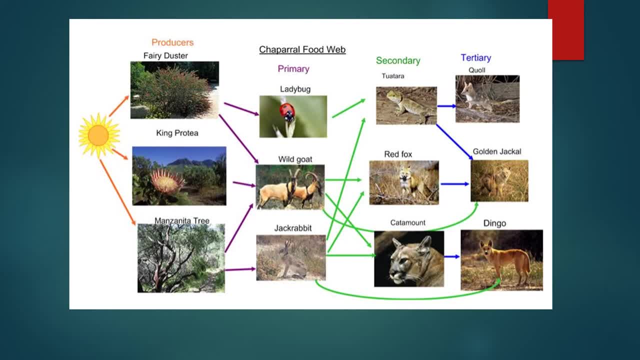 California chaparral. This is actually a Australian chaparral, So you see that it is very similar. This fairy duster here would be something considerably close to our sage. We do have manzanita trees. It's a type of like oak tree. 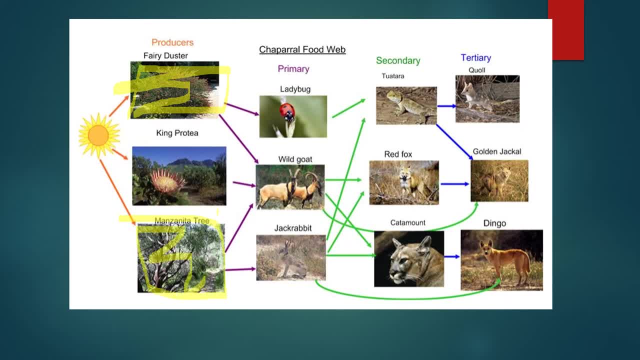 oak-like tree. So very similar, right. But then over here you start to notice things are a little bit different. We don't have catamounts. We do have California mountain lions- very similar. We don't have dingoes. It would probably be like a coyote or a smaller predator. 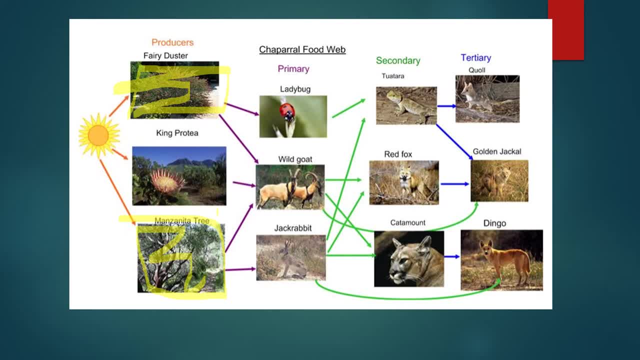 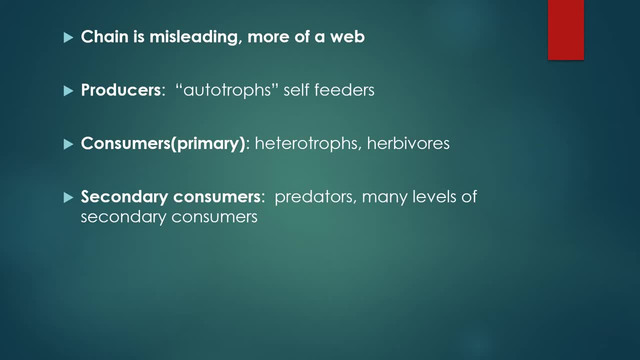 but very similar in type of vegetation, right? Okay, so this is web. A chain is a misleading term. It's more of a web. So your producers are going to be at the very beginning. These are autotrophs or self-feeders. They make their own. 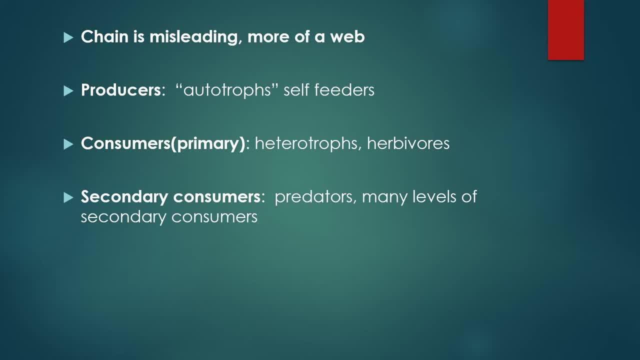 food. Those are only going to be plants, right, Also algae when we're talking about these aquatic ecosystems. but producers are self-feeders. Consumers- our primary consumers, are going to be called heterotrophs or herbivores. They only make their own food, So they're going to be. 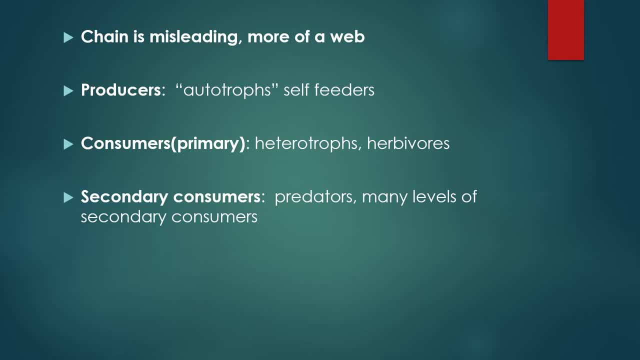 only would eat plants, right? And then again, I mean, this can go all the way to the kentary, I don't even know how to say it. The fifth consumer right: Secondary, tertiary consumers. These are predators. There are many levels of these secondary consumers. 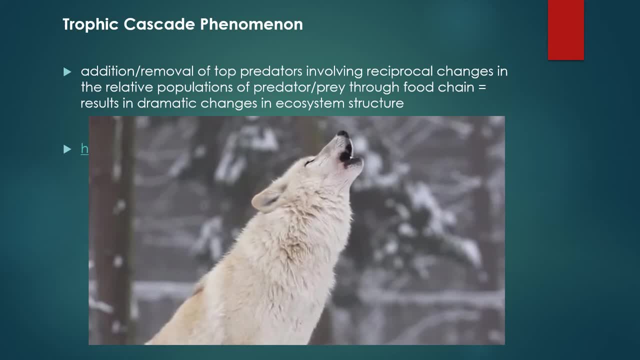 Trophic cascade. So when we're looking at this food web or food pyramid, when you introduce or remove a top predator, there's going to be a lot of different types of changes within the ecosystem, And I'm pretty sure I had you guys watch this video already. 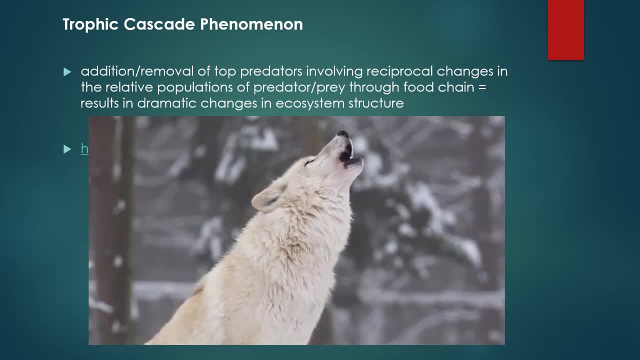 so you know right, If you introduce a top predator, your first thought would probably be like: whoa, everything's going to be ate or eaten. It's going to totally change the ecosystem, Yeah, but in a positive light. So if you remember that video- I think it was chapter eight, Yeah, 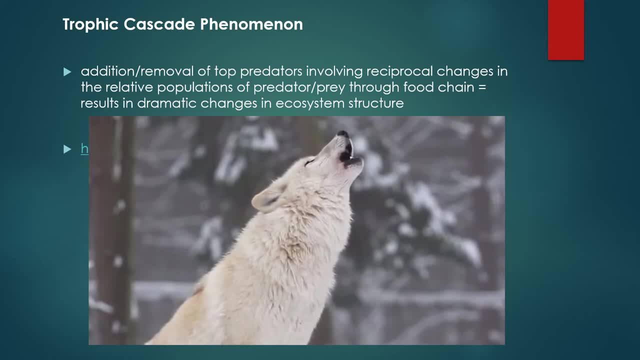 I assigned it to you guys in your modules. It has a dramatic change in the ecosystem structure, even up to the physical geography. So it's going to be a lot of changes within the ecosystem And we saw at Yellowstone the introduction of those wolves changed the meandering of those rivers. 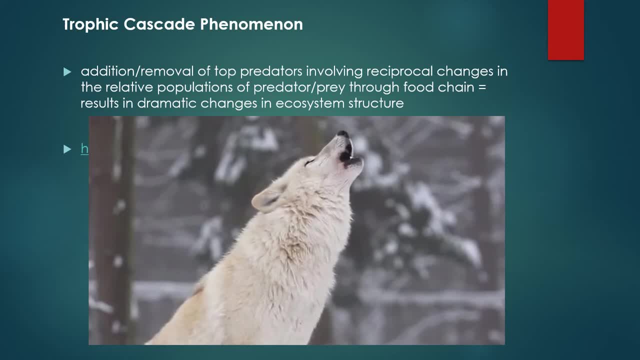 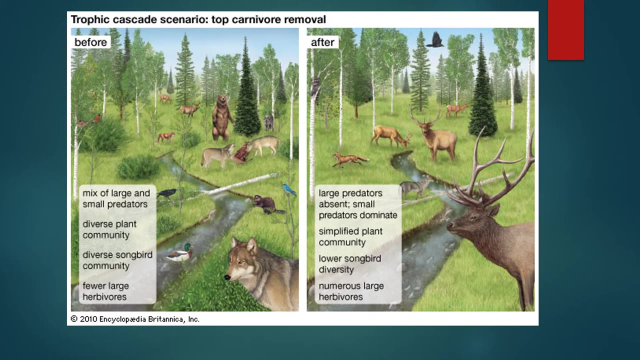 That's huge right. So an addition or removal as top predator is going to have changes in the entire ecosystem when you do do that. Here's just another scenario you have before and after. So before you have the removal of a top predator, you're going to have a lot of changes in the ecosystem And 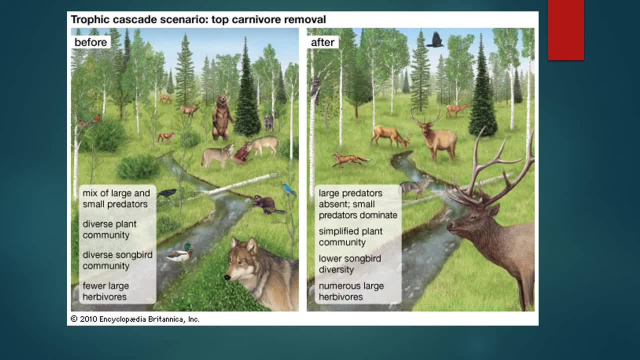 this would be kind of like the opposite. So before you remove a top predator, look at how diverse this forest ecosystem is. After, if you remove a top predator like a wolf or a bear, more so, a wolf right would be the top predator in this ecosystem because bears are more like. 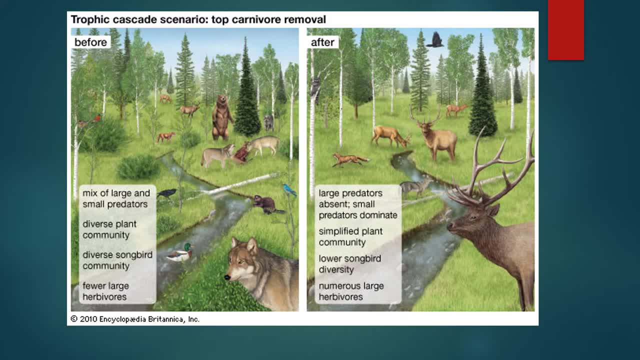 not just carnivores, So they do feed on on plants as well. If you were to remove that wolf, there's a lot of changes in the ecosystem. So if you remove a top predator, you're going to have a lot of changes in the ecosystem. 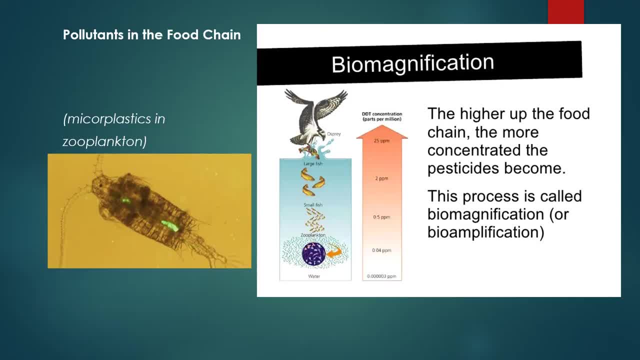 And so it's also a significant drop in biodiversity. Pollutants in the food chain, just like nutrients, water, all these things- and energy flow throughout the food chain. Unfortunately, there are pollutants in the food chain that are moving through ecosystem, I mean through aquatic food chains. 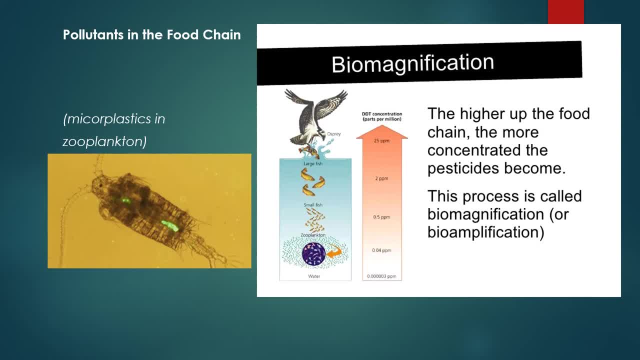 today. So we know the ocean is full of microplastics- tiny, tiny pieces of broken down plastic. They are so pervasive And so we're going to see a significant drop in biodiversity pervasive in the ocean. they have been found in zooplankton. So if you look at this picture here, 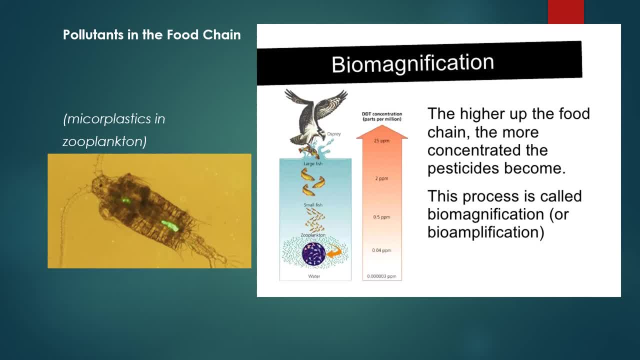 that is how tiny these plastics are. Crazy, right? So the higher up the food chain, the more concentrated the pesticides become. So what I'm going to do? what I'm going to do is I'm going to mix them all together and get the texture right. 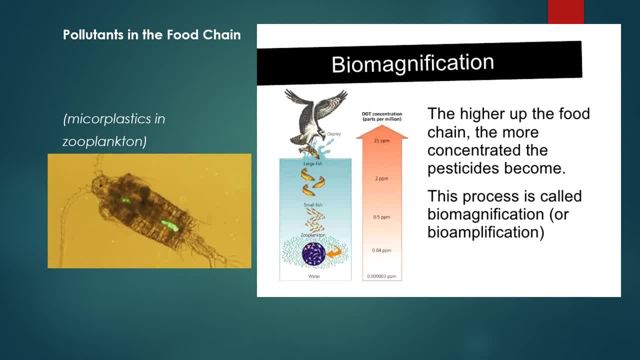 So I am going to look at the web so that I can see the biomechanical species which are actually already working on their own. So I'm going to mix these up and then I'm going to bring them back up into the sea And what you can see- what I'm doing is just looking at the 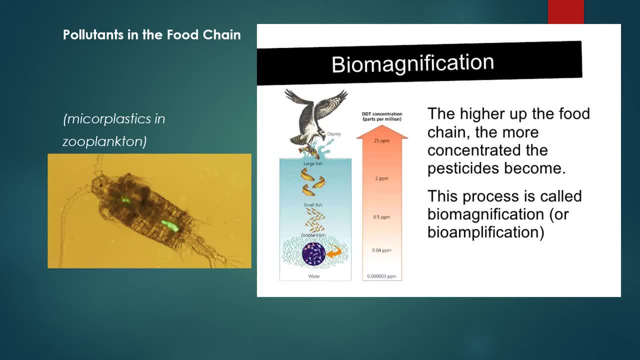 surface of this right. So I'm going to take this and I'm going to go on my flask and I'm going to put this on the other side, So you see this little thing over there. that's the water. So if you, 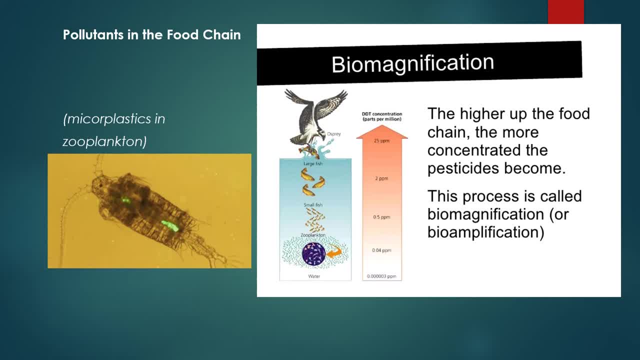 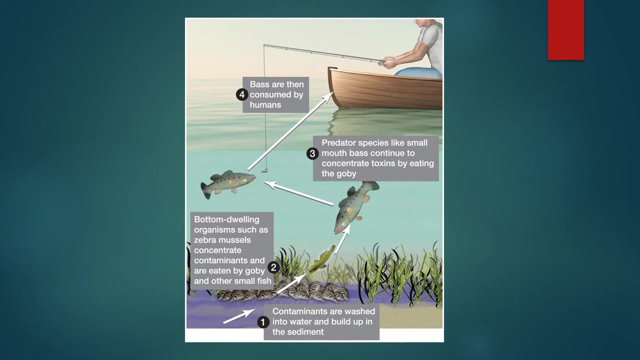 you, you, you, you, um. here's just another explanation of that: the very bottom you have contaminants, contaminants that are washed into the water. they build up in the sediment right, um. number two: your bottom dwelling organisms like mussels concentrate contaminants not eaten by goby fish. number three: 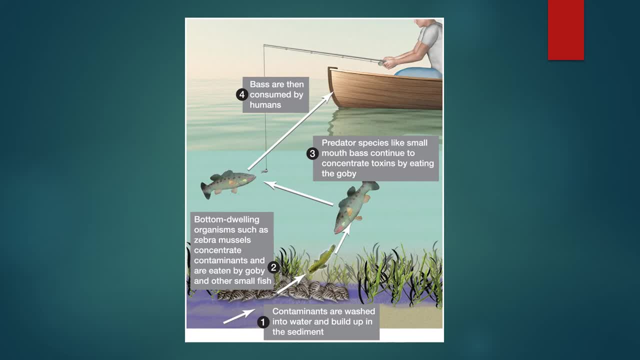 predators like small about small mouth bass continue to concentrate toxins by eating the goby fish and then the bass are consumed by humans, right? so i mean, think about of everything we try to do nowadays: eat organic, be healthy. um, look at your ingredients right. try not to eat farm-raised fish- i know that's on some people's agenda. eat wild caught. 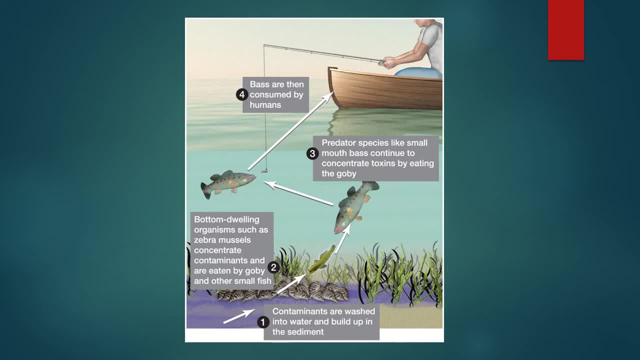 fish. but i mean there are so many instances of this. i don't know if you guys heard last year that there was a large amount of cocaine found in shrimp. that is wild, right. well, maybe not large amounts but enough to be detected. so small amounts of cocaine. 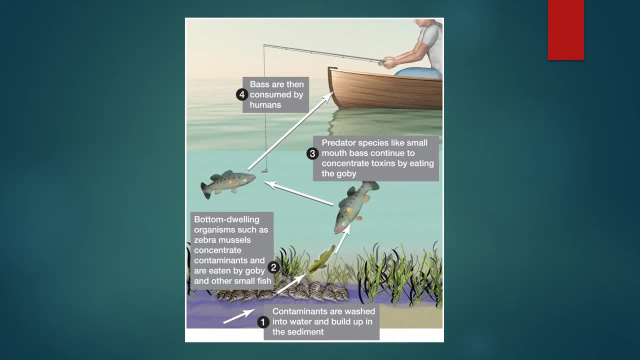 pesticides and other contaminants have been detected in uk freshwater shrimp. so i think this was last year, uh, in may, yeah, may of last year, um so. but you know, for instance, like those contaminants and shrimp are, the potential for any effect is is very low, but it just highlights the? um ramifications of pollution. pesticide use, the over, you know, production of 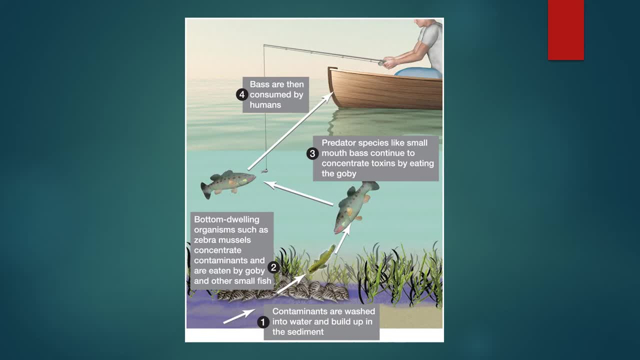 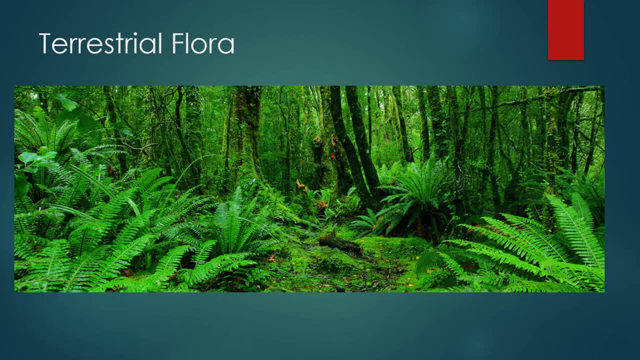 really food right on pharmaceuticals too: anything that goes down the drain is going to end up in our food. okay, let's look at terrestrial flora. um, we talked a little bit about animals. um, we are going to continue to talk about animals the rest of the chapter, but let's look at terrestrial flora. so remember flora and fauna. 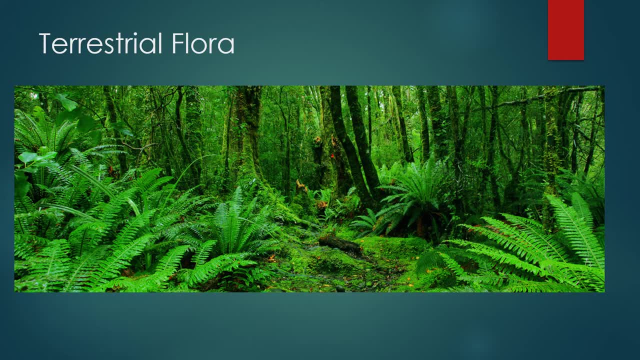 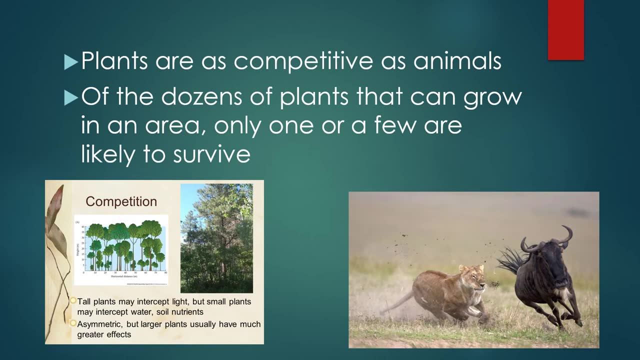 is just a fancy way of saying plants and animals. plants are just as competitive as animals. we tend not to think of them as competitive, but they are competing for things like space, light, soil, nutrients, water, especially in environments that don't have those resources, that those resources are limited. right, we like to think of animals being very competitive. they are, and i mean it. 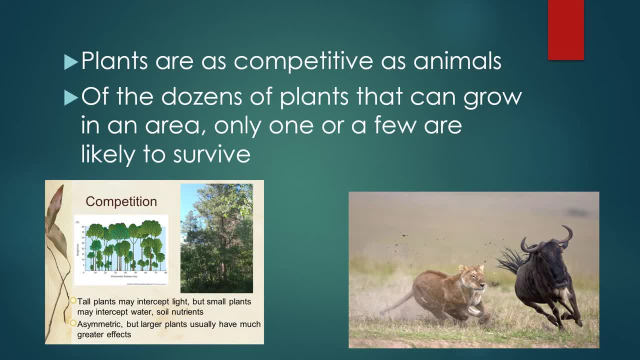 makes for a great nature documentary. right, the hunt and everything. but, just as you know, animals are competitive. plants are just as competitive. of the dozens of plants that can grow in an area, only a few are likely to survive. um, so they're always going to be competitive, but they're always going to 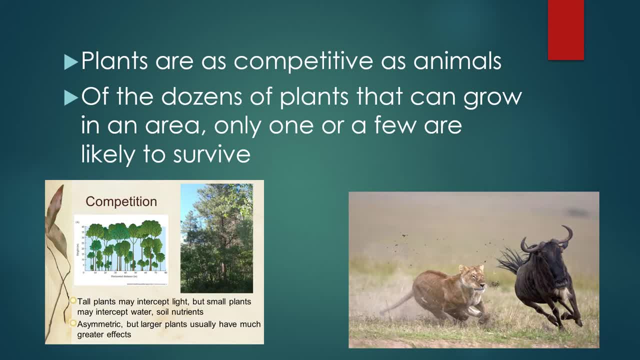 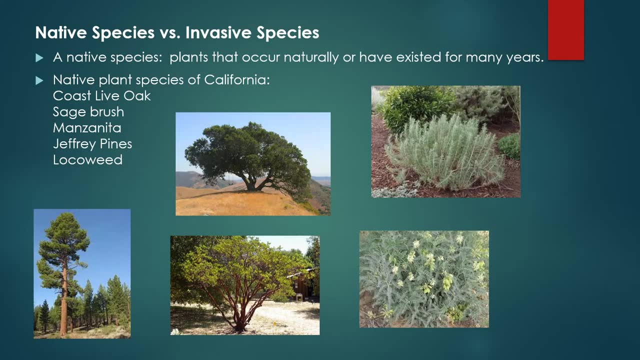 be competing for space to grow, for light, for nutrients, for soil, for water, so they're just as competitive animals. when we look at plants, there is a term that's really important for you guys to kind of understand is the difference between native and invasive species. so, native species- 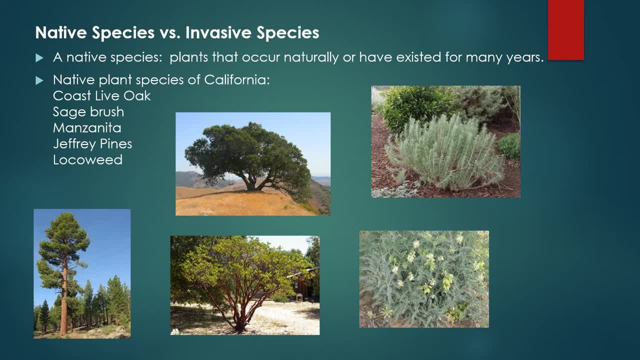 is a plant that occurs naturally or has existed for many years. when we talked about the chaparral, i said that sage was native, coast live oak was native, right? all these native plants start to bring in that natural or those native insects that bring in that native wildlife, right, it just starts. 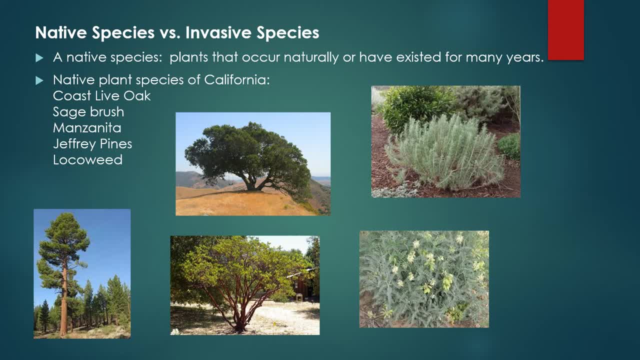 like this kind of chain. um, here are some examples of native species within our area. so you have coast live oak found in the santa monica mountains. i'm sorry, here you go. really nice, right. you have a lot of trees up here too, and some trees are. 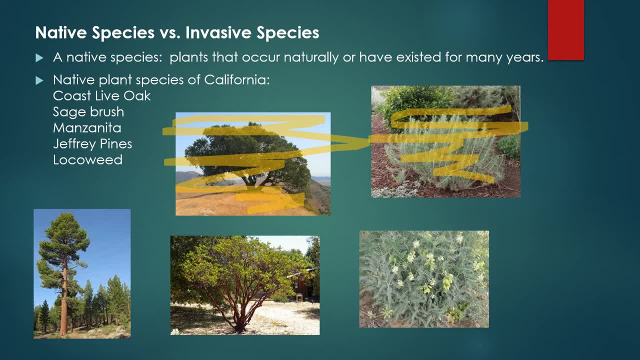 really easy to find. you can smell it on your hikes: manzanita trees, small short trees, these are all drought resistant shrubs. these are jeffrey pines, one of the only pines native to california. and this is loco weed. loco weed makes you crazy, i'm just kidding, it's just called loco weed. 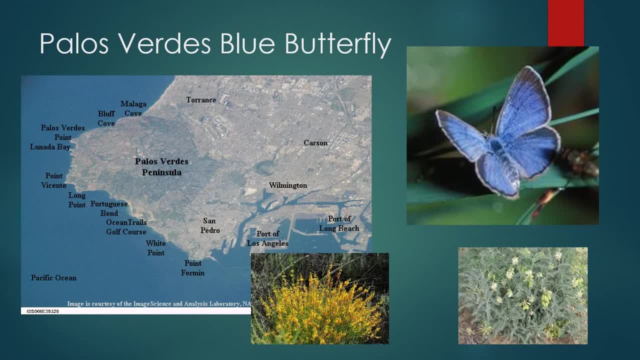 So the importance of local weed, for example. this is a very small example. This is a Palos Verdes blue butterfly. They thought it went extinct and you know, when it's a tiny animal like this or a tiny insect, it seems not to get the attention that, like a rhino, would get right. 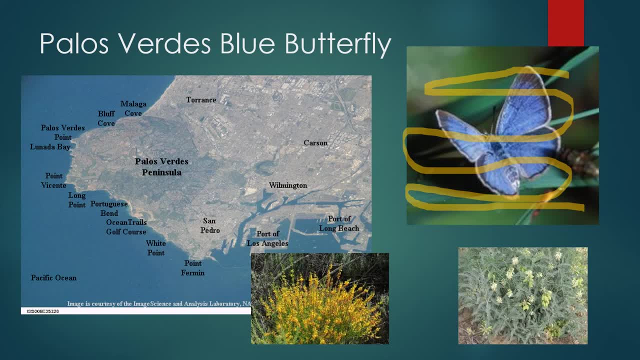 or like tigers, would get right. They get all that attention because there's these huge beautiful animals- And if you saw that movie Racing Extinction, they explained that very well- Like a tiny brown bird. nobody seems to care if a tiny brown bird or a tiny butterfly goes extinct. 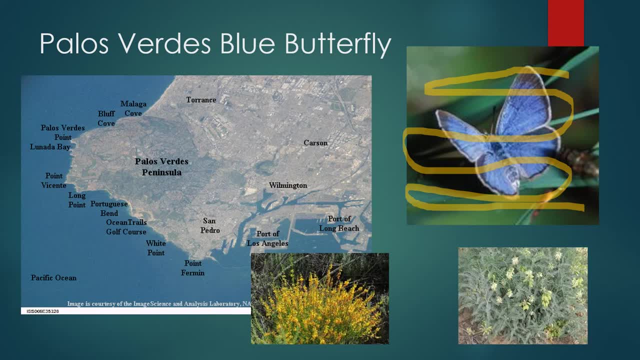 So they thought that this scientists thought that it was extinct. but in 1995 they went out because they're only found in the Palos Verdes Peninsula. They went out and actually found one and it is very localized because it can only live where there is deer weed. 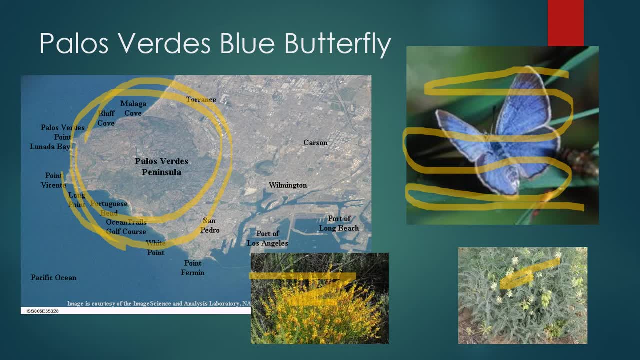 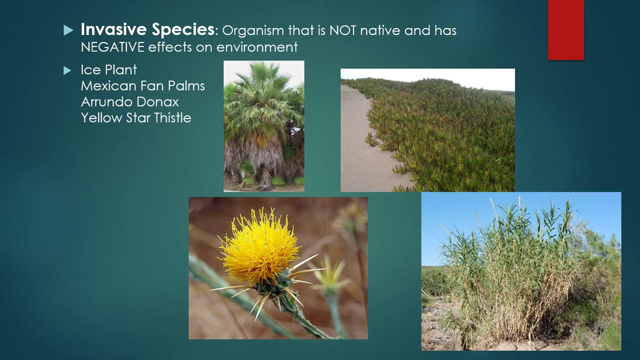 or local weed. So it's very, very endemic to the peninsula of Palos Verdes. So that's just an example of how our native plants foster the biodiversity of an area. Okay, so we talked about native species, and what I want you guys to understand is: 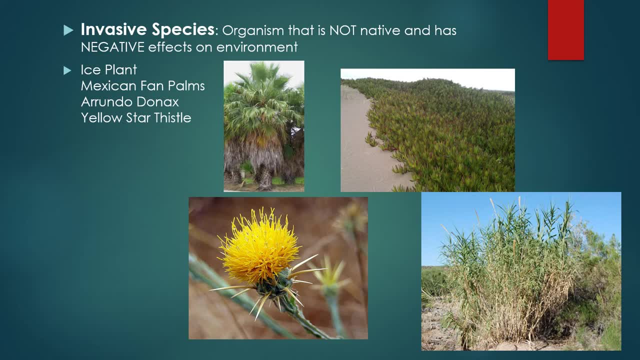 that an invasive species is not only just from somewhere else or not native, but it has a negative impact on the environment. Okay, so you can very well have a plant that is not from the chaparral and it grows well, but it's not invasive- An invasive species. 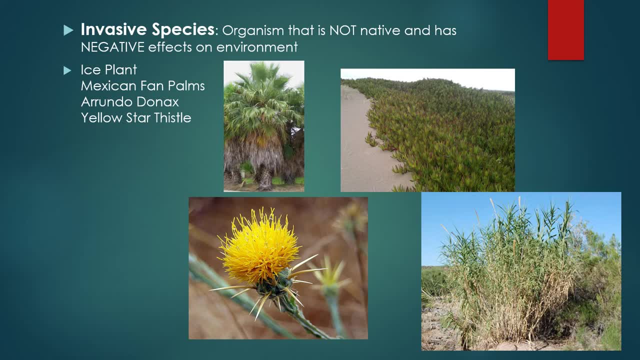 will have a negative impact, meaning it will overcrowd or it grows too quickly and takes out that natural vegetation Or, for instance, like an invasive species, will have a negative impact on species or exotic species of bird is just going to eat everything, right, has a negative impact. 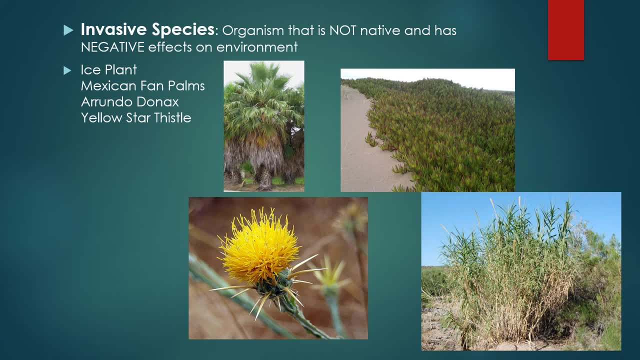 so you can have a natural plant, a non-native plant, and it grows well and it doesn't have a negative impact. that's fine. but an invasive species has a negative impact, for instance, ice plant. that's this picture here um mexican fan palms. these are not native and they're invasive. 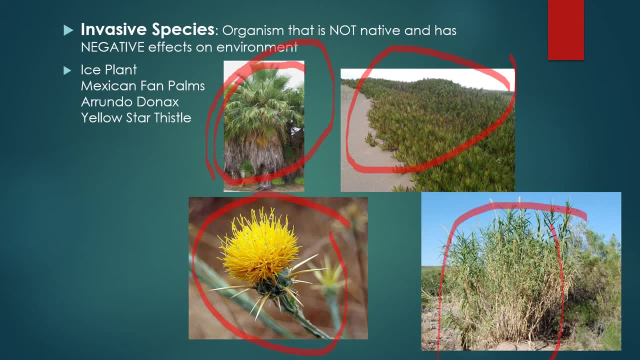 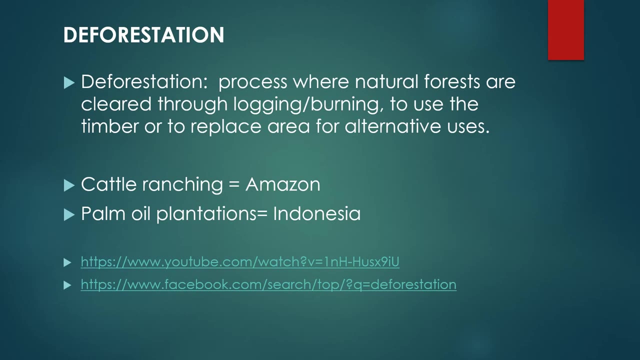 yellow star, thistle, arondodonax- i'm sure you guys have seen all these. maybe you don't even notice plants, but i mean these are really common in southern california: deforestation- when we're looking at forests, deforestation is just where natural forests are cleared through logging or 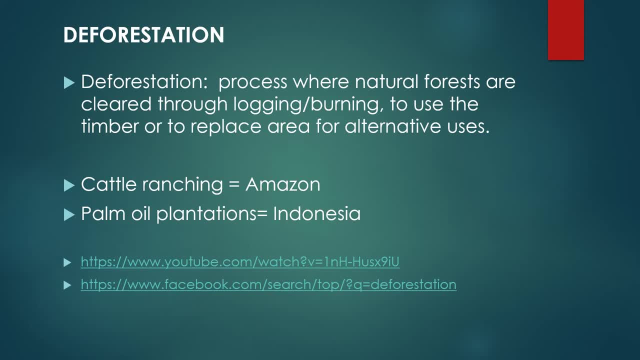 burning to use the timber or to replace that area for our alternative uses. the main driver of deforestation is going to be agriculture. the main reason we are burning and clearing all our forests is not for timber, it is for land use. so either to raise cattle or to, to grow feed for cattle or to. 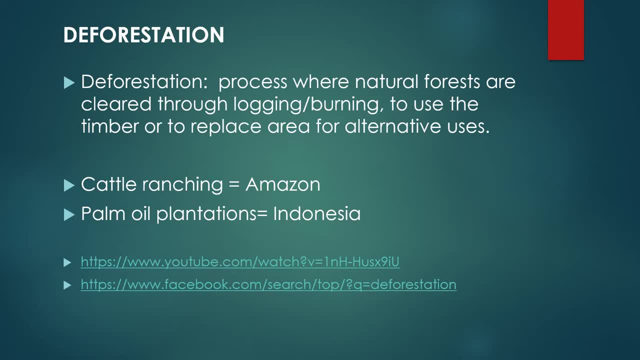 to raise livestock or food for us. that is the main reason we are clearing our rainforest. in the amazon, cattle ranching is a main reason. in the late 90s it was soy, soybean plantations. i can't talk today, soybean plantations, um in indonesia it's palm oil plantations. so you know, it's not because we're 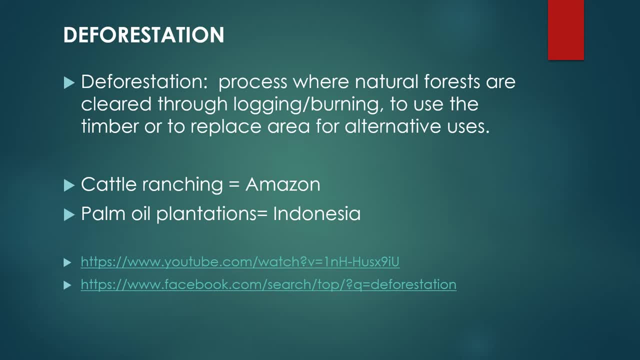 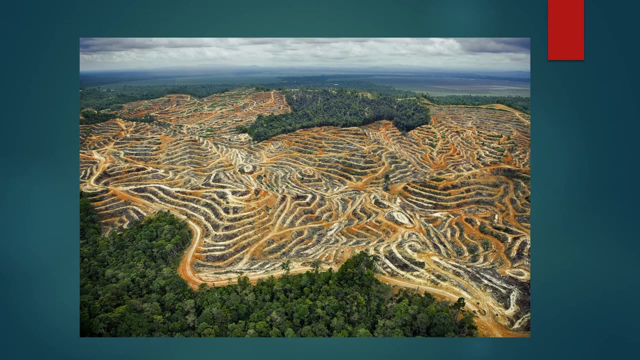 chopping down trees to make paper out of them, right. that was like when we were little. that's what we thought. save the trees, it is really for our food- for food. that's the main reason. so here's just a picture of deforestation and how pervasive it is and how it separates ecosystems- right, if there is. 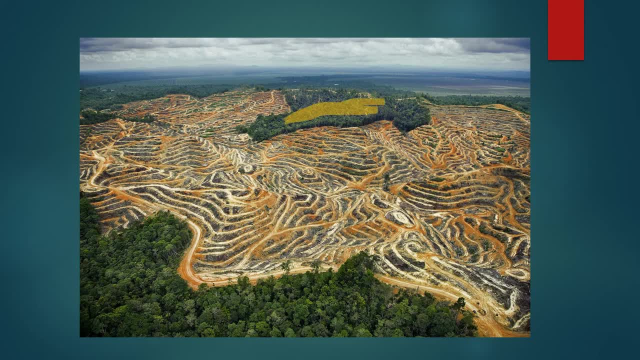 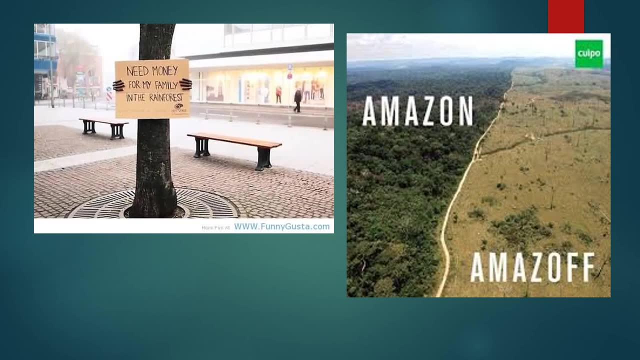 i mean any type of wildlife left over here. how will they get over here, right, if that is their reality? so these are just pictures i thought were kind of sad and interesting. right, need money for my family in the rainforest. this picture here, okay, so let's look at terrestrial. 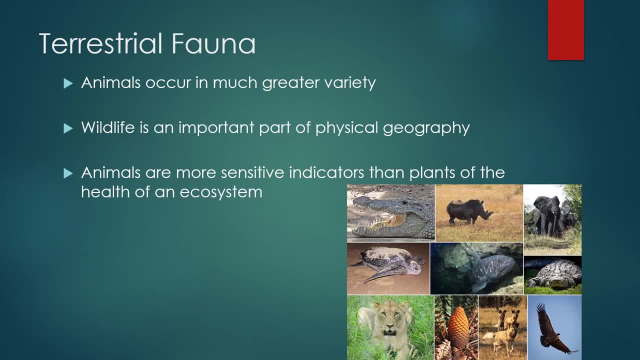 fauna moving on from land, from plants, to animals. terrestrial fauna occur in much greater variety. there is many more animals than there is plants on earth. wildlife is an important part of physical geography because, as geographers, yes, we're looking at the landscape, but we're not ignoring 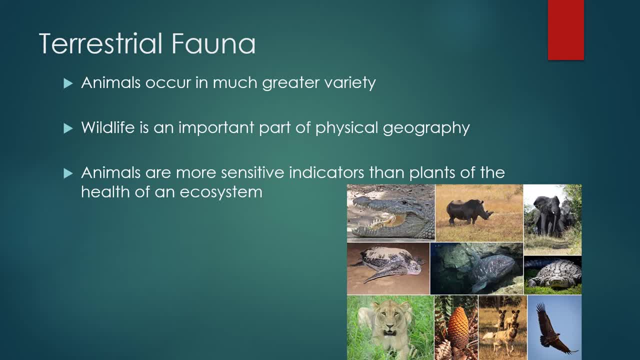 what is found on the landscape. right. animals are more sensitive indicators than plants of the health of an ecosystem. why? because animals can just leave if there is a change within the cosmic situation. an ecosystem is not providing the resources an animal needs, they'll just go look for a new. 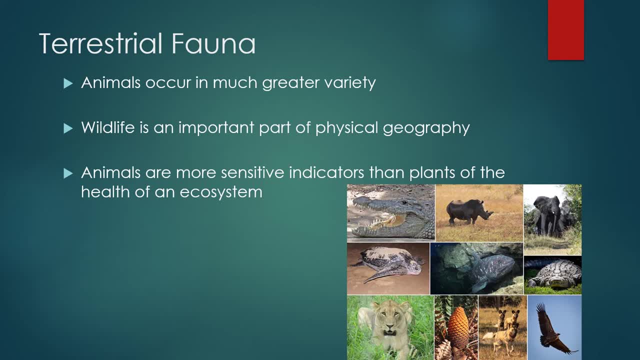 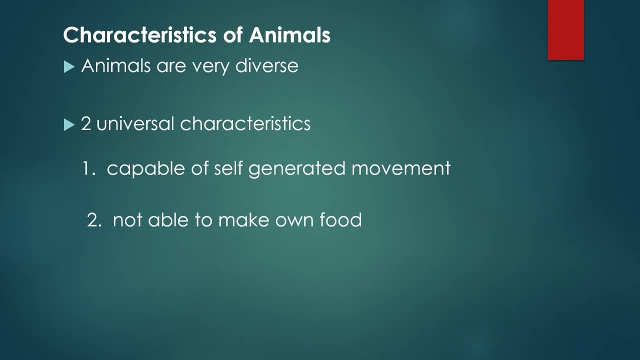 ecosystem. unlike plants, right plants have to stay. obviously they can't get up and walk around. right plants will have to stay and try to hack it out or, you know, just survive through the drought or whatever. it is that that ecosystem is characteristics of animals. they're very 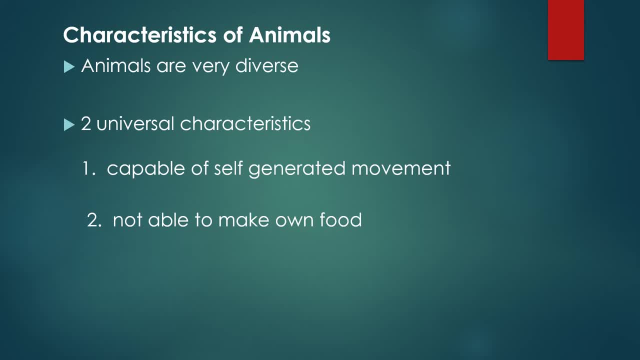 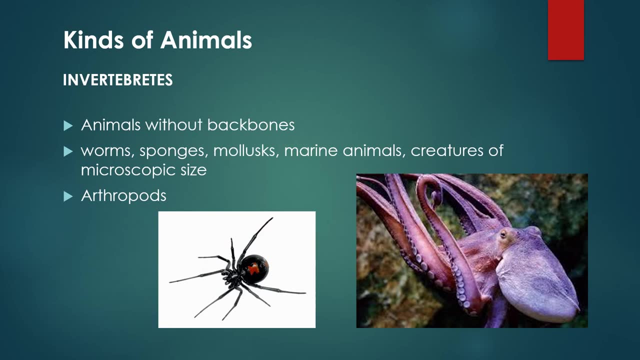 diverse. you have two universal characteristics: they're capable of self-generated movement and they're not able to make food. different types of animals you have invertebrates. these are animals without backbones, worms, sponges, mollusks, marine animals, creatures of microscopic size and the 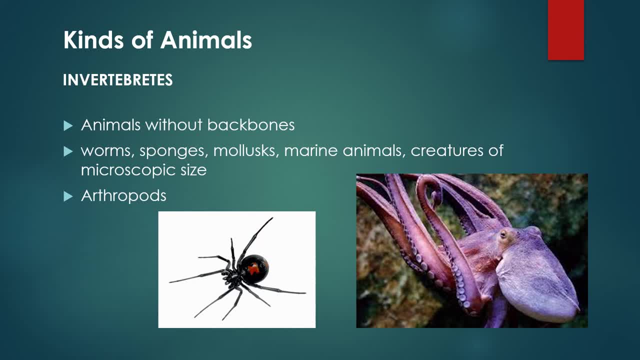 largest category of invertebrates are arthropods. these are spiders or insects, right? so the reason i put a black widow picture there is because i was born with a black widow and i was born with a bit by a black widow twice in one day on my thigh when i was 16 years old. it crawled in my pants. 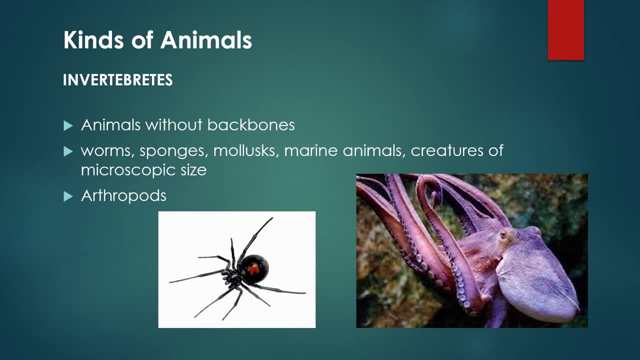 when i was using the restroom and as i pulled up my pants i felt fire on my legs. and then i grabbed something and i kind of like smushed it between my fingers through my jeans and i looked and it was a black widow that i remember trying to kill earlier when i was cleaning the restroom. 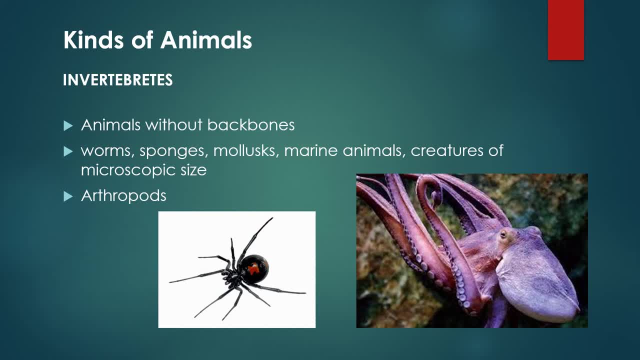 and i stayed the night at a hospital. they didn't have the anti-venom so i had to go through these like body aches. they said it was going to be worse than labor. i remember everything hurt and then they gave me morphine and i will never forget what that felt like when the morphine went through the 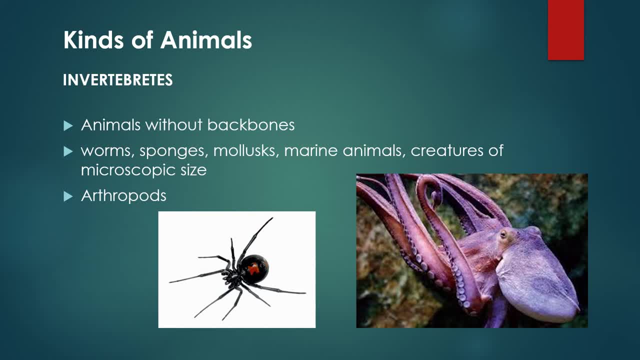 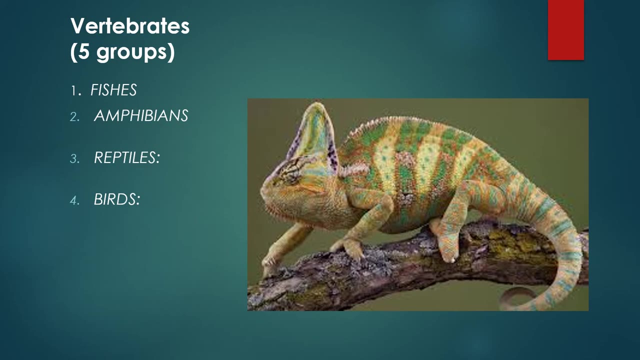 iv system. yeah, it was pretty traumatic, but hey, i'm alive and i'm not afraid of spiders anymore. um, so here's your little story for the day um. vertebrates, these are animals with backbones. okay, so you have fish and there's five types: fish: amphibians, reptiles and mammals, but there are. 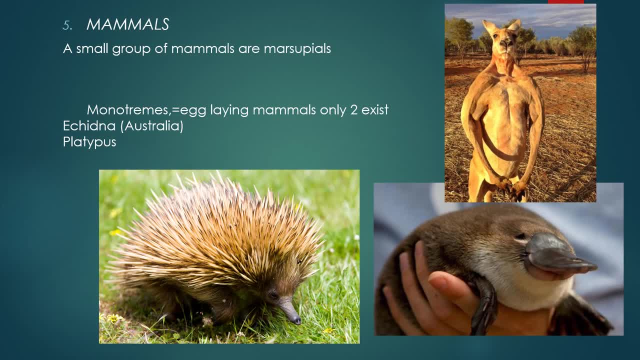 so what mammals do is that they give birth to live young. that is one of their characteristics. another one is that mammals can take, have true hair, not just whiskers. so there's a few, well couple, animals in the world- or mammals, sorry, in the world- that do. 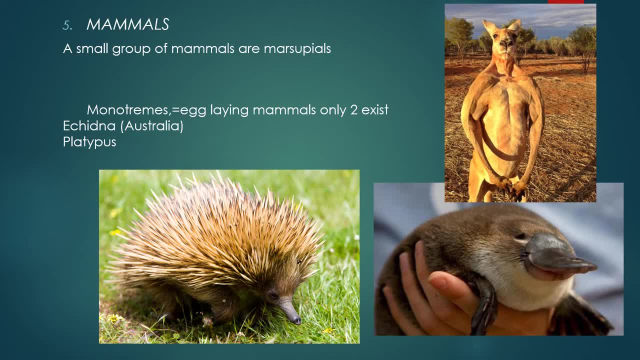 lay eggs, but they are still mammals. these are called monotremes, egg-laying mammals um only about two of them exist um an echidna and a platypus, and there is a small group of mammals that are marsupials. so marsupials have two different phases. 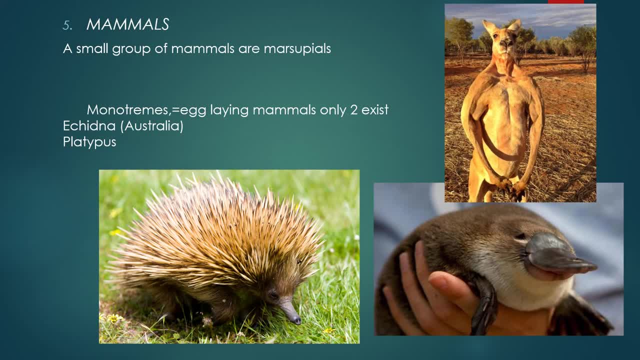 when they're giving birth. so, like when the like, for instance, a kangaroo, is a marsupial, the kangaroo will have, like, a baby inside her pouch and, um, she'll be pregnant. so she, she has two different types of milk, she lactates two different types of milk, one for her baby inside. 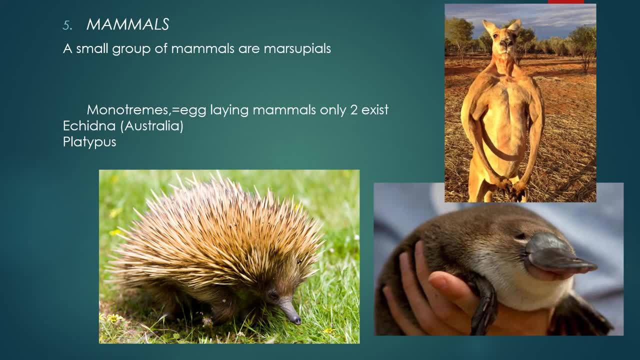 her pouch and then if she has a baby outside of her pouch, it's really weird. she's like pregnant nine years of her life. it's really interesting the way that happens. and, um, the reason i have this jacked kangaroo here is because they do fight. they fight each other and they box each other. 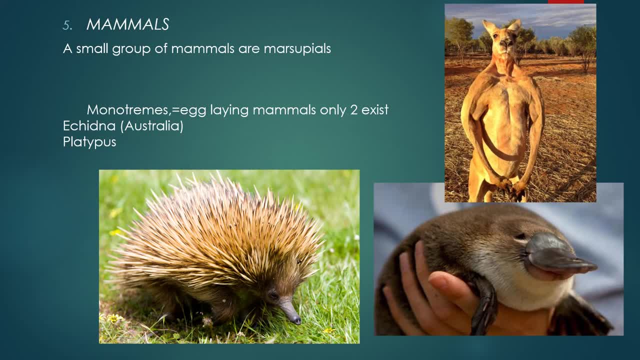 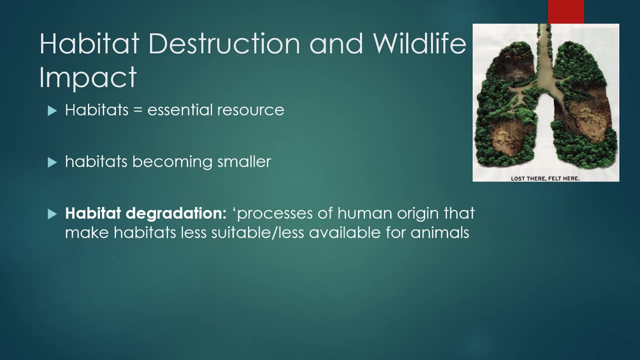 for a fertile female. isn't that cute. it's kind of like what you see at the bars right in downtown fullerton. just kidding, all right. so habitat destruction and wildlife impact: what are we doing to wildlife, right? what are our impacts on wildlife? obviously, habitats are an essential resource. 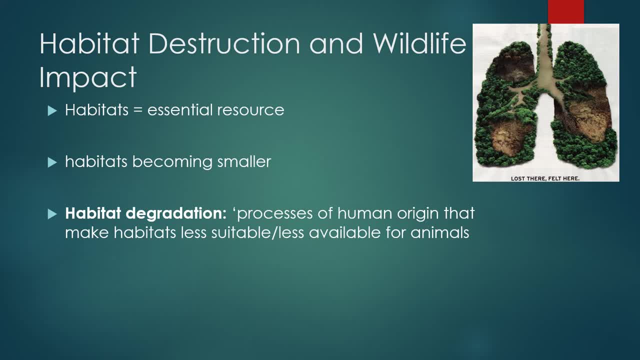 but unfortunately habitats are becoming smaller and smaller. i mean, i just showed you the picture of deforestation. that that's just one example. right, we see that in these rainforests, but even somewhere even closer, like here in southern california or california, we are impacting these habitats as we go along. 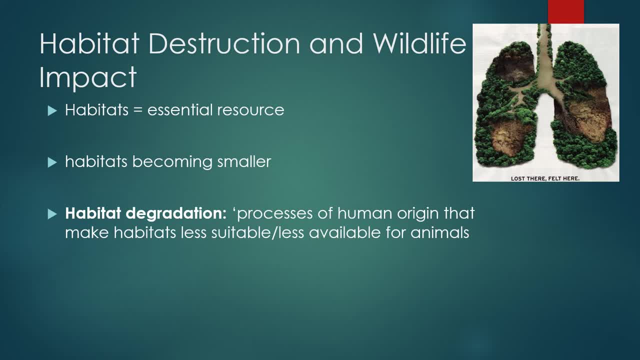 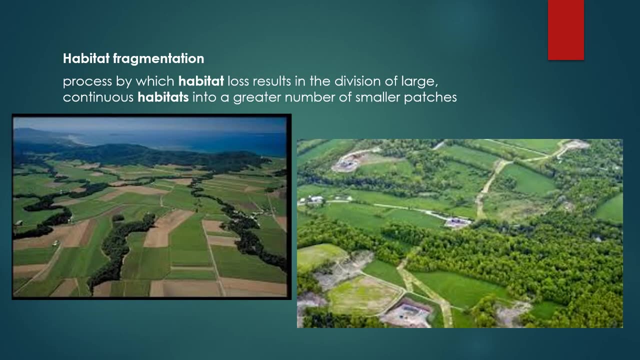 as we start to sprawl outwards and develop more and more because there's more and more people right, habitats are becoming smaller. habitat degradation is a process of human origin that makes habitats less suitable and less available for animals. habitat fragmentation is a process by which habitat loss results in the division of large 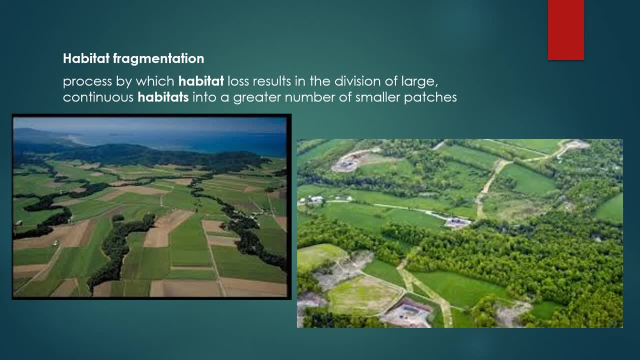 continuous habitats into greater small patches of habitat. so this picture here illustrates a great example of uh, a healthy habitat, like here with the wild snake. and now here we have a little bit more details of what habitat loss is like. we have a population of eight million in our state and we have about 100,000 animals in our state, and the area is about one billion inhabitants and a population of 117 million are living in the state of california, and we are coming up on a population size that is almostمuch. there is no, it's a population size that we have. you know, it is not much, so we're going to have to. but we have to do a little bit of a study of it. so i am going to look at that and then i'm going to look at this and i'm going to focus on a question that comes from, a question that comes from one of the both of our people who are asking us to discuss- and i'm going to give this a chance- people who are 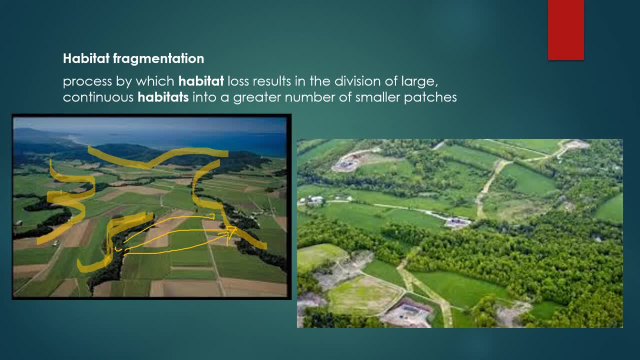 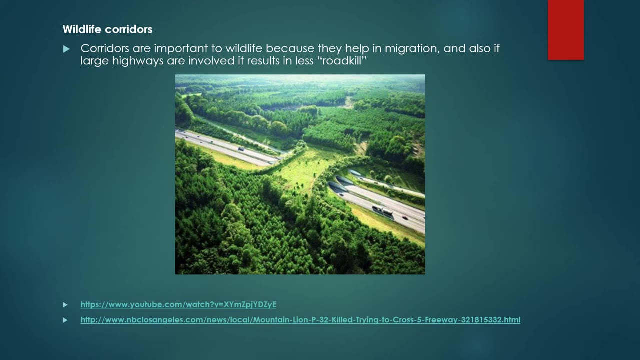 to mate right. So that poses a big problem if there is, for instance, a large highway running through this area. So there has been something developed. This is kind of like good news. We usually don't have good news in these classes. These are called wildlife corridors. They are 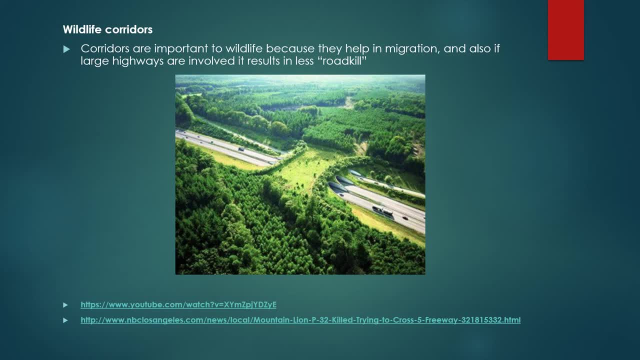 developed specifically for wildlife to take, instead of using the roads and becoming roadkill. right Corridors, wildlife corridors, wildlife passages, eco ducks- They have many different names. They're important because they help in migration and looking for food, And you know. 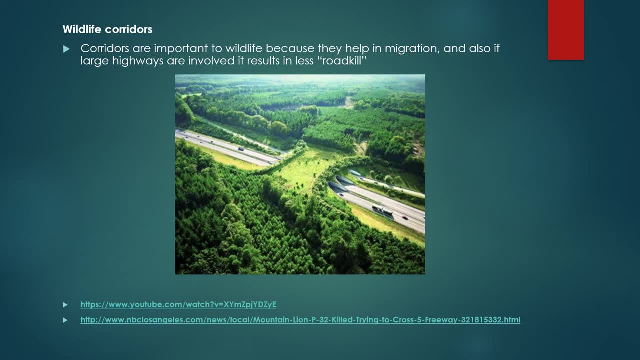 I have a lot of students that ask like: hey, do they really use them? Yeah, they really use them. They just go by scent, right, So they would take it, And we see them all over the world and they do help. So that's kind of cool, right. 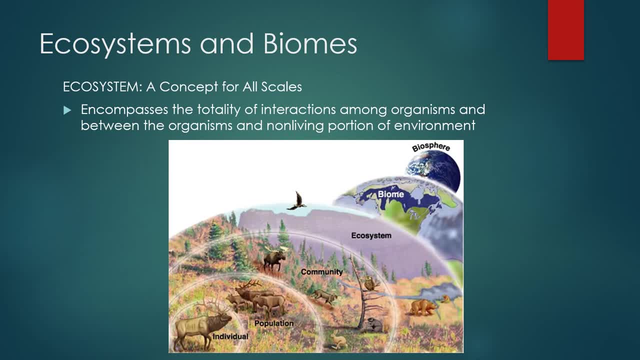 Okay, last part of today's lecture. I am going through it very, very quickly: Our ecosystems and biomes. These are just scales at looking at our biosphere. right Overall, we would call the living portion of the planet the biosphere, but we can break it down even further. So I love this picture. 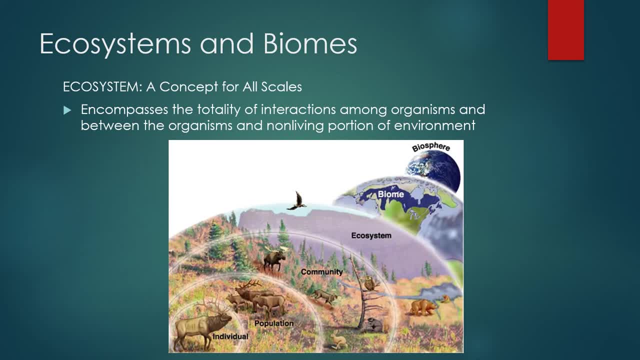 here because it shows how every- it's like the Russian doll effect- right, You have the individual species. That individual species is part of a population. You have the individual species, right, Still the same type of animal. Then you have this population of elk or whatever living. 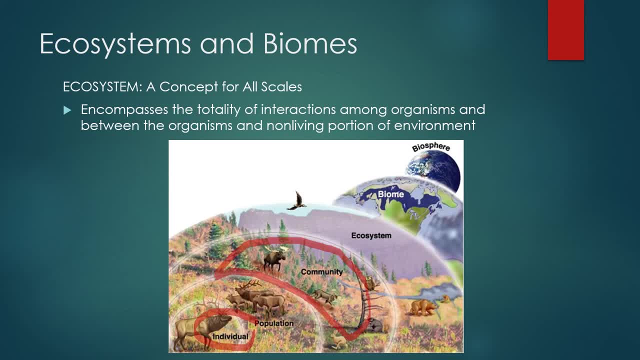 in this community, different types of species. right, Then this community exists within this ecosystem, even larger. Now you're looking at not just the living, but you're looking at the non-living portion too, Then this ecosystem belongs within this biome, right. And then the 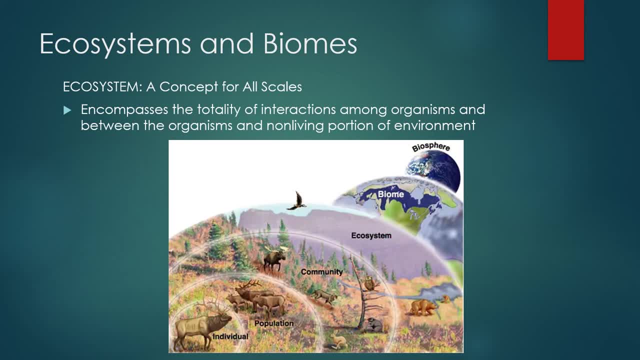 biome is found within the biosphere, So pretty cool way of looking at the living and non-living portions of the planet. And then you have this population of elk or whatever living in this living portion of the environment. Why are ecosystems important? Why is it important to? 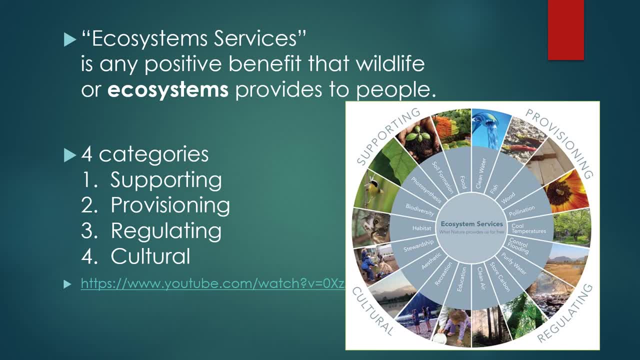 save them, to preserve them, to conserve them, to fight for them. So most of you would say, because it's our duty, We're called to be good stewards, right For future generations, So my children's children can experience them. Yes, those are all correct answers And that would be like the romantic side of it, right Like the flashback. So I would say, okay, we're called to be good stewards. right Like the flashback. So I would say, okay, we're called to be good stewards, right. 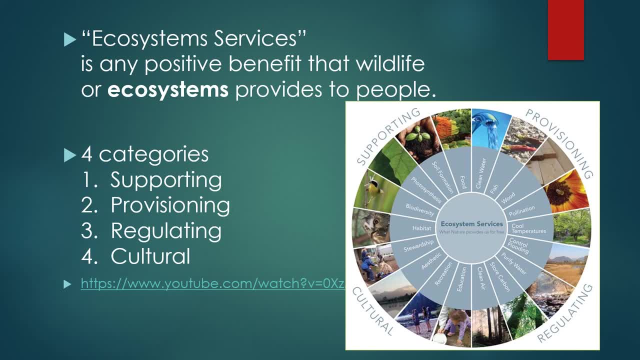 Like the flashback. So I would say, okay, we're called to be good stewards, right, Because we're. Oh, because it's beautiful, Earth is amazing And yeah, I mean that's like why I got into this field, right. But if we want to implement the conservation of these ecosystems into public, 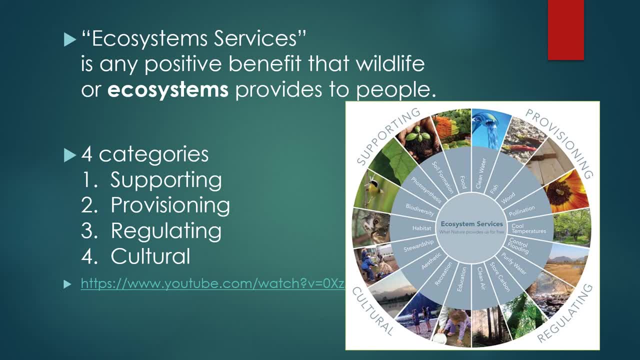 policy at all. no senator or you know nobody in office is going to listen to you and say, because it's beautiful, You kind of have to attach these benefits or services that these ecosystems would provide. and then you attach monetary value and say like, hey, if we preserve. 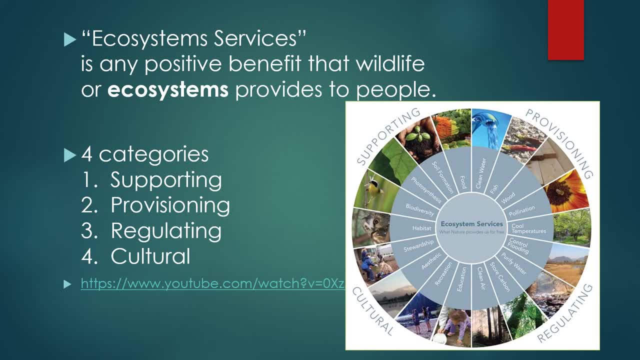 this park, then we will save this much money in medical bills because less people will have asthma and that's like i'm overreaching, but that is like a really good example of why you need to find benefits to these ecosystems, because unfortunately, humanity, we don't listen to things if it's not. 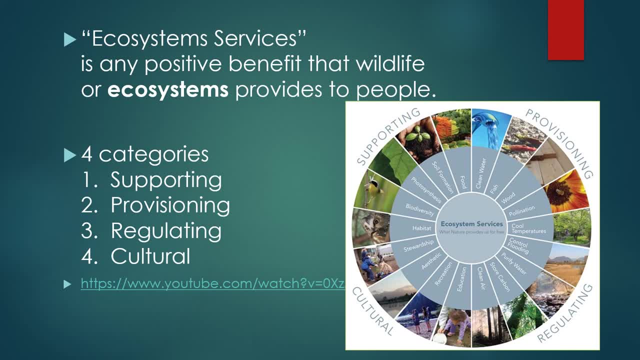 beneficial to us, right? so what do ecosystems provide to us? these are called ecosystem services. it's any positive benefit that wildlife or ecosystems provide to people. so it could be a supporting service, could be provisioning, regulating, cultural. so supporting would be like photosynthesis, creating food, soil formation, right, provisioning services would be like fish. 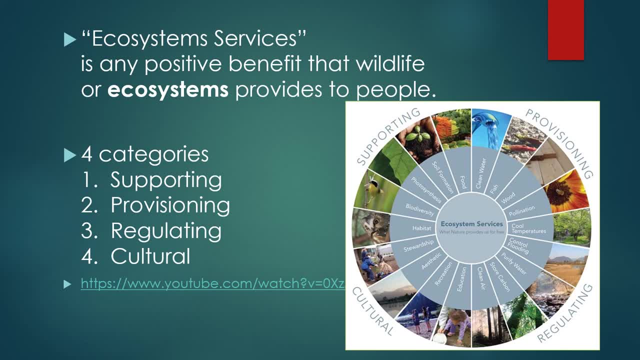 pollination, cooler temperatures, because i mean the more parks we have, the cooler the temperatures are. these are called microclimates, regulating services. so trees store carbon, they clean our air, they purify uh. water can be more pure. you can control flooding, flood mitigation, clean air- all these things there are regulating services and cultural. 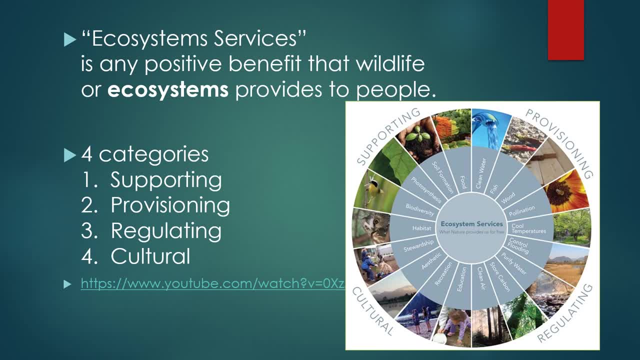 that's like the flowery side right, recreation, aesthetics, stewardship, education. so these are all reasons we should protect our ecosystems because they benefit us, right? i mean, at the end of the day, that doesn't sound nice to me, but if that's how we're going to have these people in office, listen to us then. 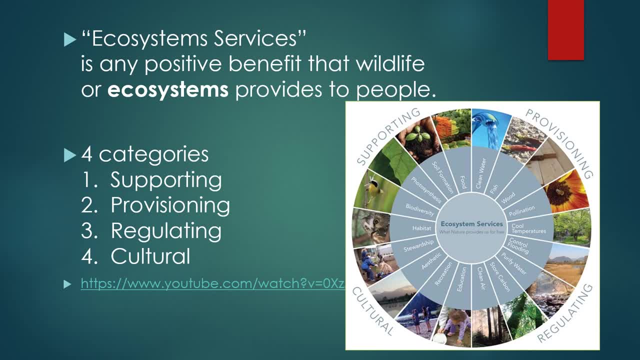 i mean, that's the way it should be right. in other countries, though, this is a little bit different, because other countries rely on eco tourism. people are going to mexico, for instance, to look at their beaches or the volcanoes, or going to um like the bahamas right or anywhere really in the caribbean. 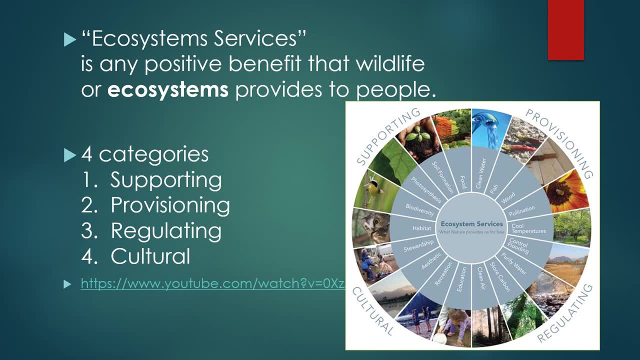 they rely mostly- 90 percent now maybe even more- on tourism for their economy. so protecting these ecosystems and these wild areas are much, it's much more valuable in other places in the united states, right um, i don't think people care about the environment at all in the united states. i mean you can just by the way our economy is run. 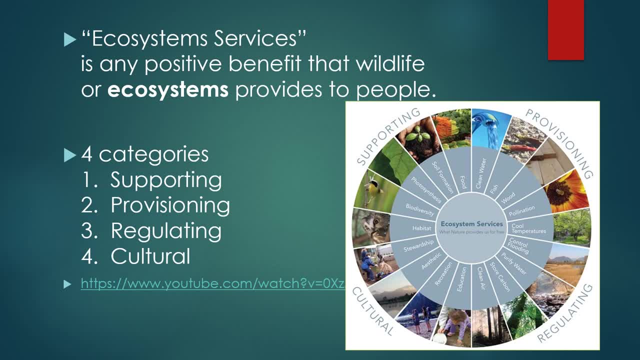 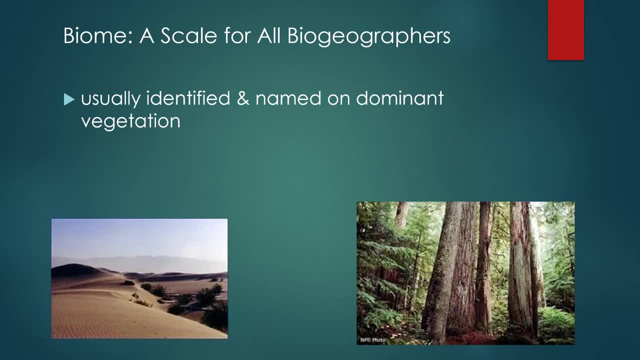 we know that capitalism, greed and fossil fuels is really what runs the economy. but i digress. so let's look at a larger scale: biomes. this is how we're going to look at the entire planet, based on vegetation type. so it's really the type of vegetation there is and we're looking at. 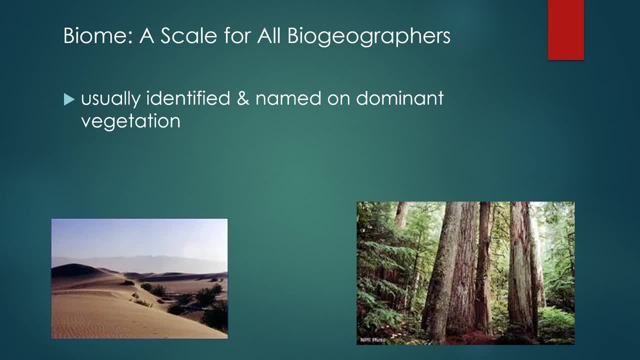 different varieties and patterns and kind of breaking down the planet into different biomes. so it's usually named and identified on dominant vegetation, but we're also looking at the animals within that biome too, right? so if you were to take my environmental geography class, we would have a whole week of presentations and you would have your own biome and we would get 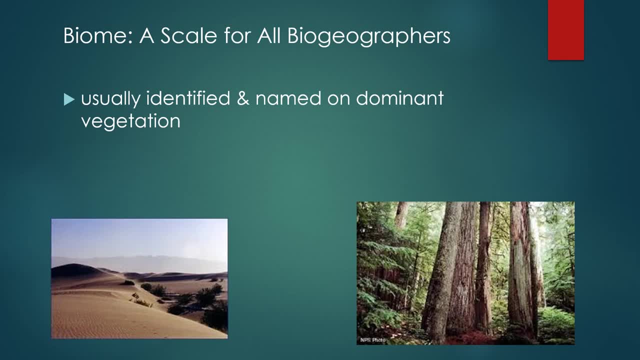 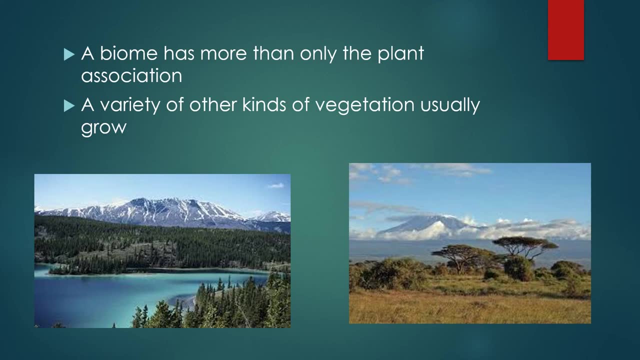 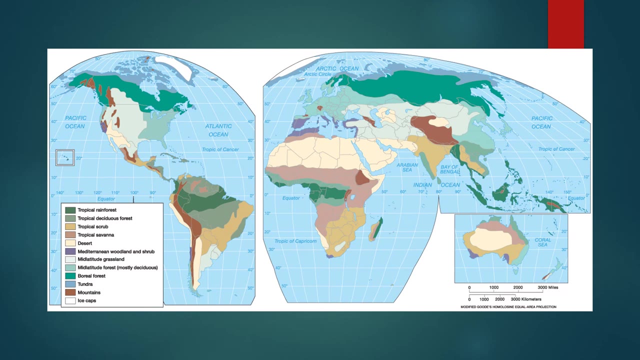 really in depth on it, but i'm just going to go through this pretty swiftly. um, a biome can have more than one plant type. you know other types of vegetation do grow, but there's kind of like this dominant type of plant within the biome. so here is your different biomes. um, obviously we're not ignoring climate or 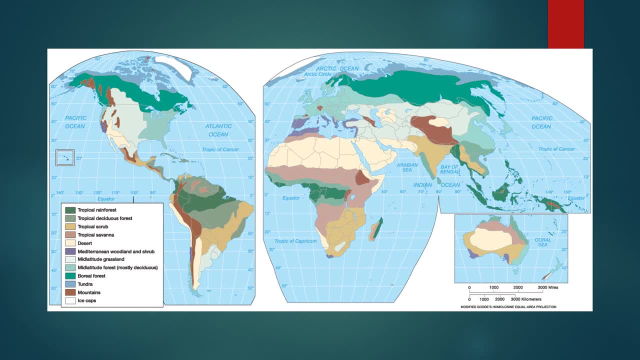 precipitation, because our dry areas with low precipitation are going to be our deserts right places with higher precipitation. you're going to have more vegetation, maybe more of our forests, not just rainforest, but there's like tropical rainforest, there's a deciduous forest, there is a mid-latitude forest, so it's kind of 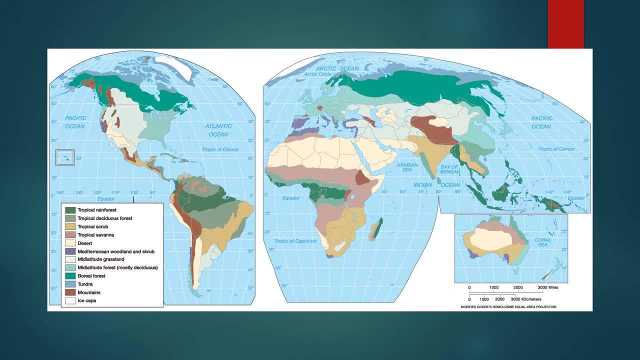 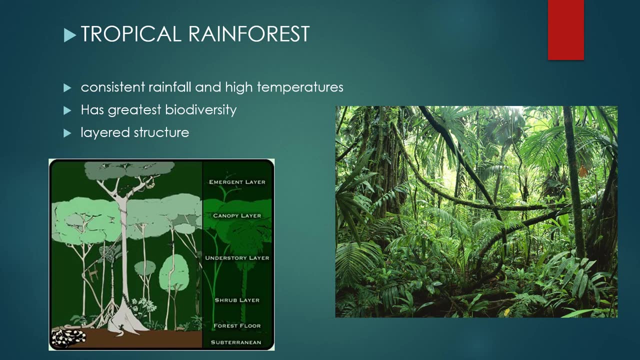 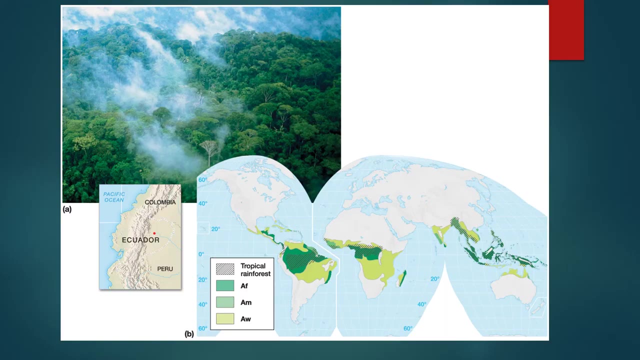 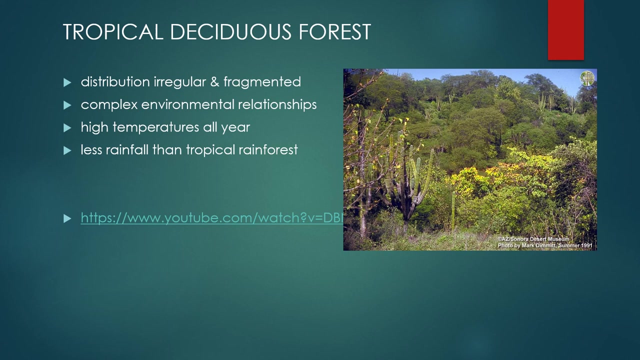 um, just different for latitude. right, your tropical rainforest is where you have the most precipitation out of all: biomes: consistent rainfall, high temperatures, great biodiversity layered. stranger, this is where it's found: tropical rainforest, tropical deciduous forest. now you're moving away deciduous forest by the name. you know you are still within the tropics, right. however, there is. 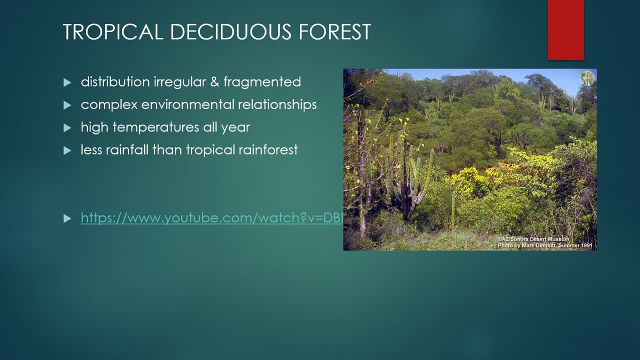 less rainfall. now here you have deciduous trees. deciduous trees lose their leaves in climatic changes or seasonal changes. right, unlike the tropical rainforest, you're not going to have trees that lose their leaves in the winter or fall, or the fall or winter, so tropical deciduous. 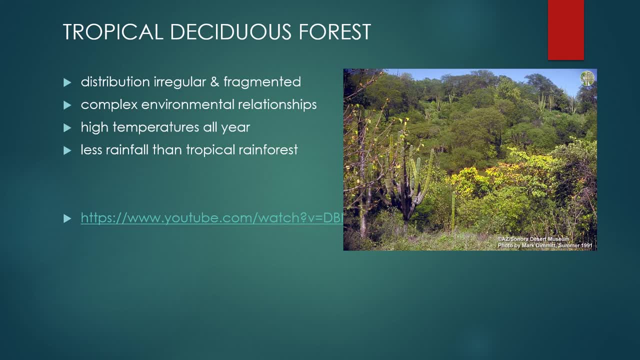 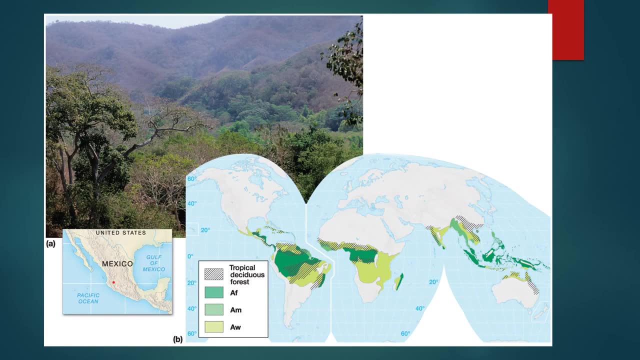 forest. you kind of have like this mixture of both, giving you a complex relation: environmental relationships, high temperatures all year. so this is where you would find it, kind of on the outskirts of the tropical rainforest. so you're moving away from the equator, you're still in the tropics. 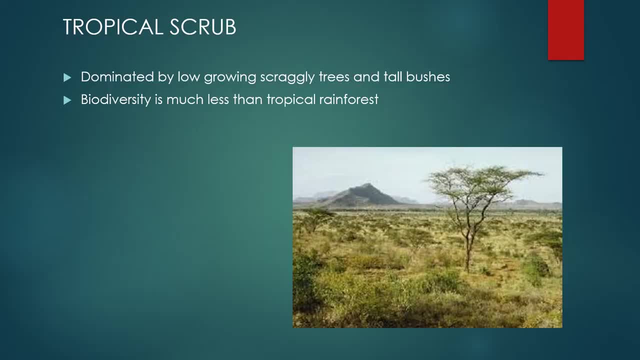 tropical scrub. you're moving even further away, on different sides of the continents, and you're going to have much more dry conditions, but you kind of have this mixture of low growing, scraggly trees, tall bushes. you have your dry season and a mild wet season. so it's going to be quite different than your tropical rainforest, but it's still within the 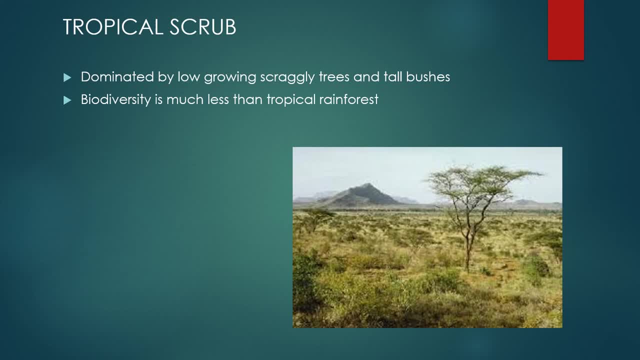 tropics. this is very much close to your mid-latitude scrub, which is going to be like your chaparral. so you're looking at the name and it'll tell you where it's located. right, there's a tropical scrub and there's a mid-latitude scrub very similar to the tropical rainforest. 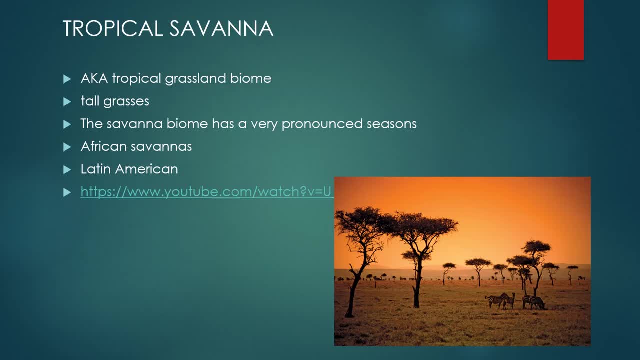 tropical savannah. these are going to be grasslands. there's a tropical savannah. there's also mid-latitude grassland, which are going to be your prairies. so grasslands are obviously lots of grasses, right? so these are tall grasses. the savannah biome has pronounced seasons. you have your very wet season. 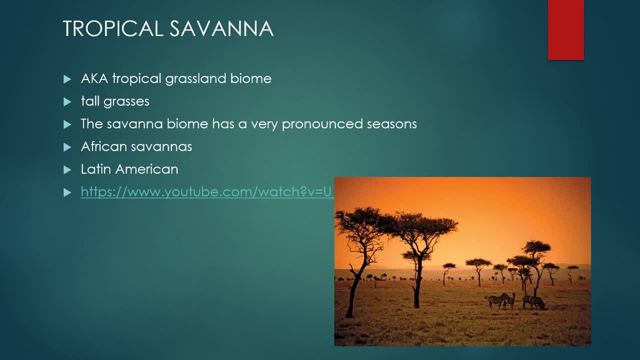 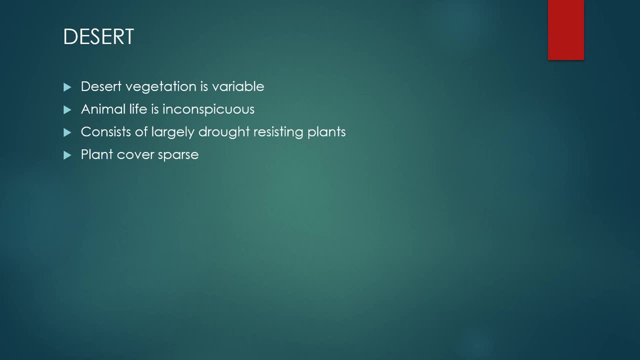 and dry season. you have two types of savannas: african and latin american savannahs. this is where they're located, and then the desert is going to be your very dry biome. plant cover is sparse. desert vegetation is variable, lots of drought plants. this is one of our largest biomes. 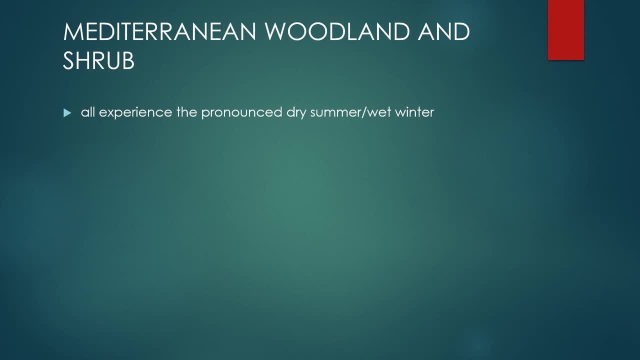 mediterranean woodland and shrub. this is the biome that we live in here in southern california or los angeles, the um, the name of the climate zone is mediterranean, but the name of the climate zone is of the biome is Mediterranean woodland and shrub. they all experience the 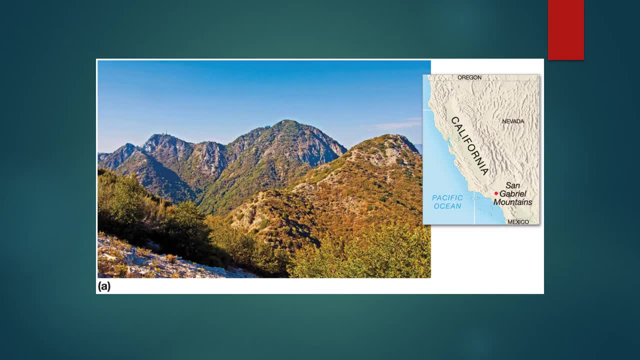 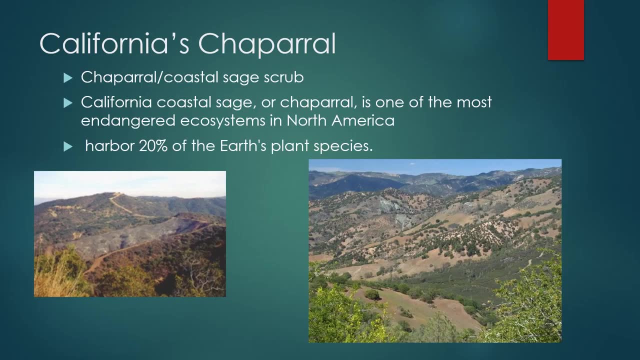 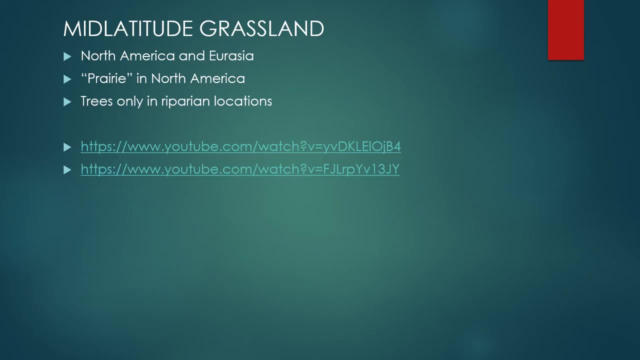 pronounced dry summer, wet winter, then that's where that's located, very, very small in terms of California, Chaparral. I gave you guys a huge lecture on this in chapter 8, so this is probably the same thing though: mid-latitude grassland, North America and Eurasia. in North America it's called prairie, so this is where. 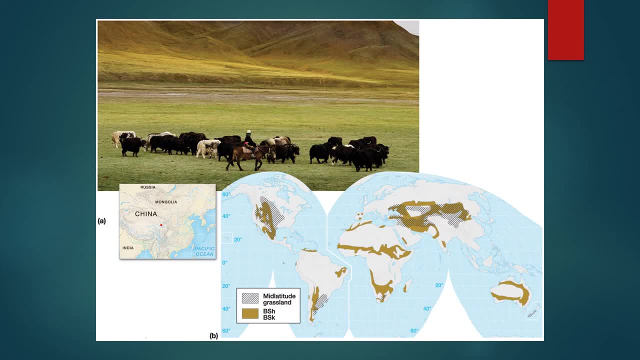 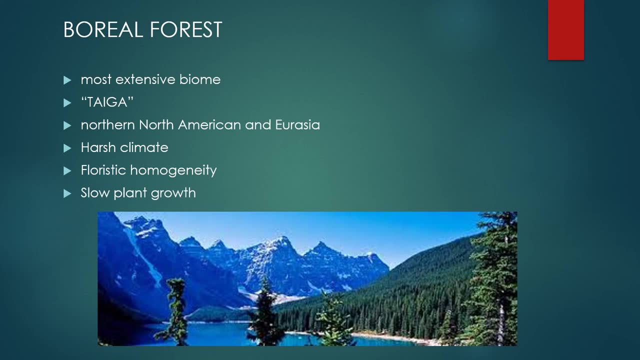 it's found parts of Mongolia, North America and your boreal. this is the most extensive biome, also known as a taiga. this is on the fringe of- oh no, no, sorry, I meant something else- North America and Eurasia, so parts of Canada and Russia. harsh climate, very cold, but not cold enough to where. 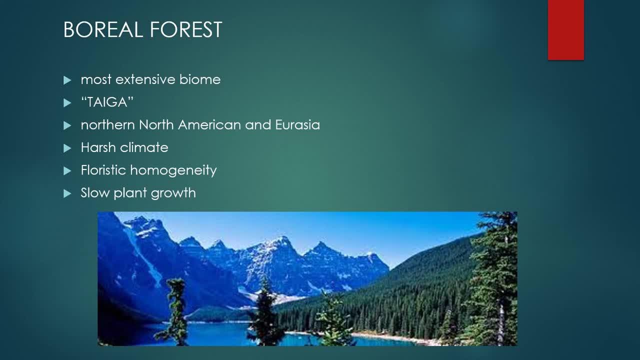 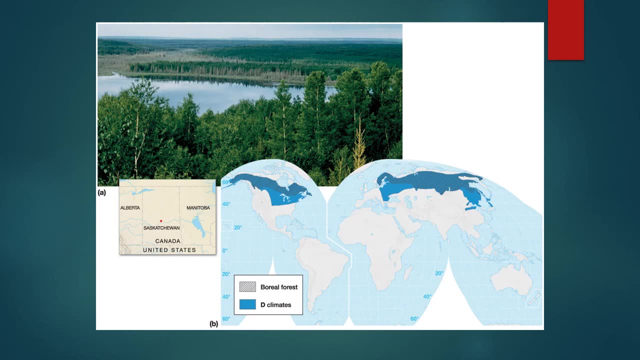 there's no plants, so floristic homogeneity, which means the same types of trees. really it's just gonna be coniferous trees, pine trees, slow plant growth. this is where it's located, all in the northern hemisphere. why? because at these latitudes there's no land in the southern hemisphere, and then the tundra. there's a cold desert, or 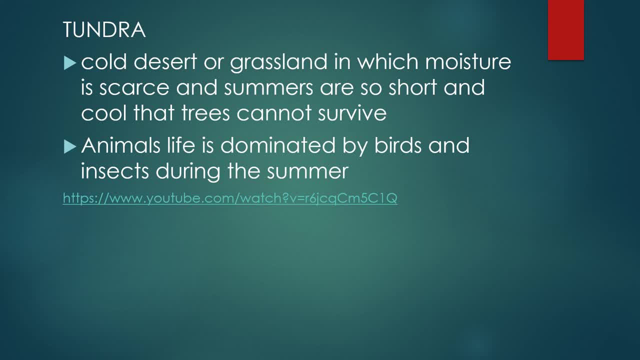 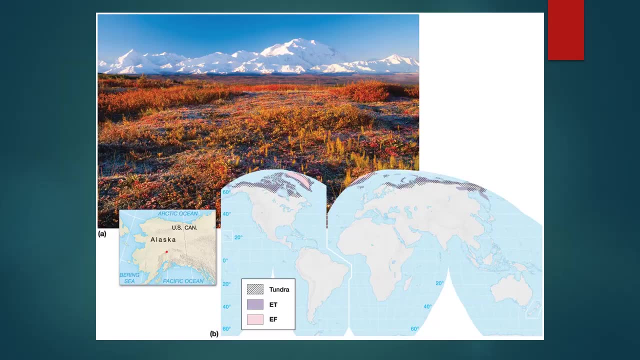 grassland. moisture is scarce, summers are short, trees cannot really survive. you really just have lichens and mosses. that's a good thing about it in the tundra, and this is where it's located, just at the very, very top of the boreal forest. so that's about it.